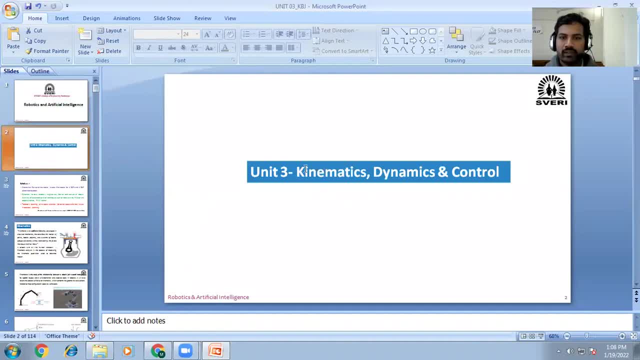 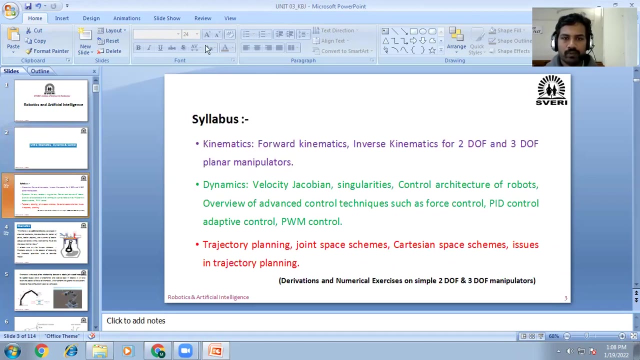 Okay, the subject title is sorry. unit title is: Kinematics, Dynamics and Control. Okay, out of that. In previous lectures we have covered the Kinematic part, Dynamics only this Trajectory Planning. okay, this part is remaining from our third unit. 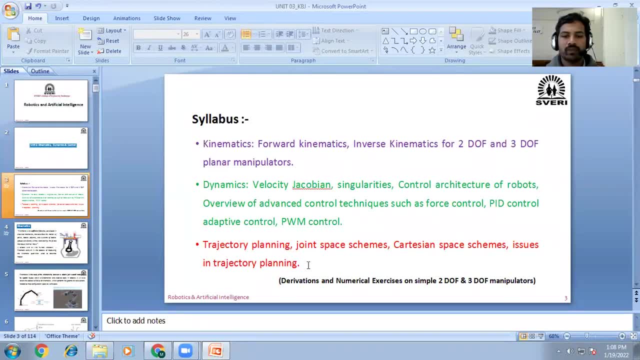 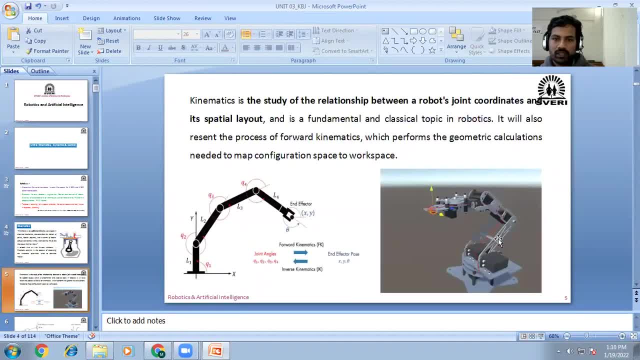 In Dynamics we have seen the Forward Kinematics, Inverse Kinematics for 2 degree of Freedom and Planar Manipulator kinematics- okay. after that we have studied a kinematics- forward kinematics and inverse kinematics- okay. in forward kinematics we are finding the end effector position- okay, suppose. 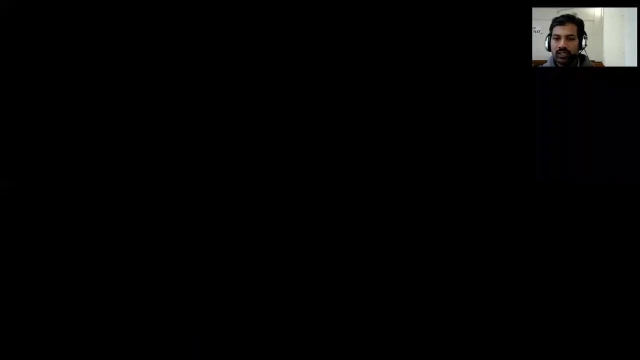 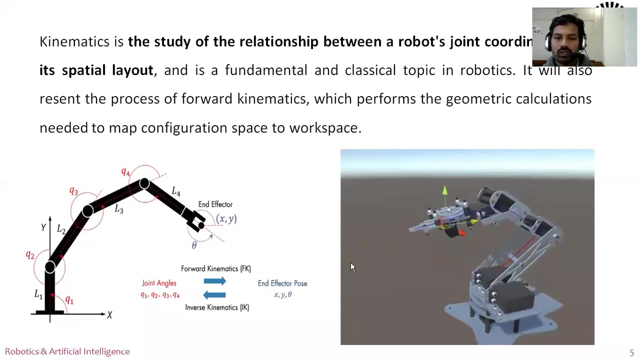 you want to find the end effector position, in that case we are using the okay, this position from the base. if you want to find, find out of this robot, then in that case you can use this forward kinematics and in inverse kinematics we are finding the angles of joint angle of. 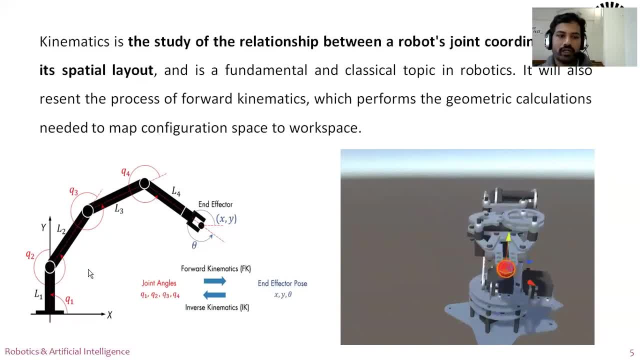 each link, okay, protect links upon joint angle. find out: okay, suppose this link number one and the link number two, okay, the angle it is made by these two links are the q2. okay, and if you see, with respect to base, this link number one has, uh, has a angle of q1, okay, 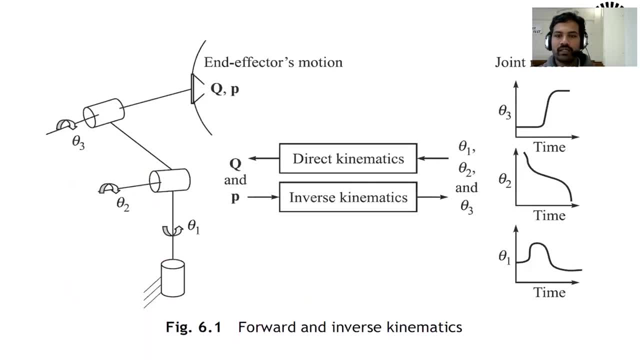 okay, now this already we have discussed again. uh, direct kinematics, that forward kinematics also it is known as a direct kinematics. okay, you might be in exam, might be you confused what you mean by direct kinematics, kinematics, forward kinematics. okay, direct and forward, both are same one. 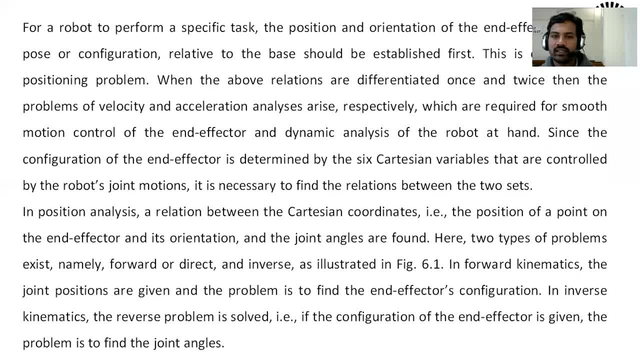 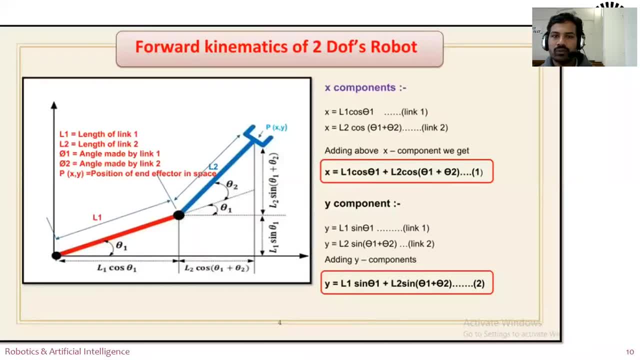 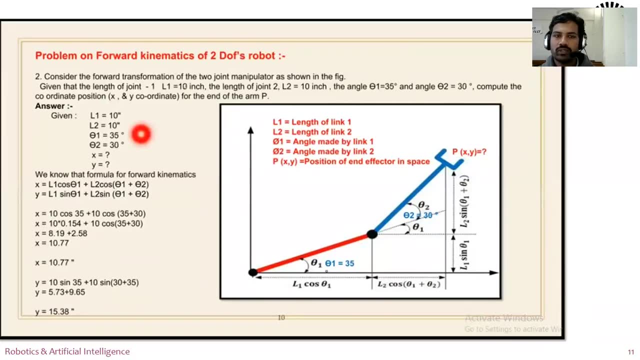 okay, there is only word. differences are there? okay, we have seen the. what is mean by forward inverse kinematics? okay, again, we have seen the derivation of forward kinematics of two degrees of freedom- robot problem. we have seen next problem on forward kinematics of two degree of freedom. 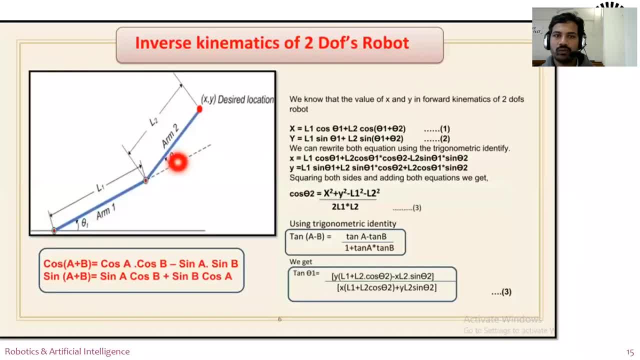 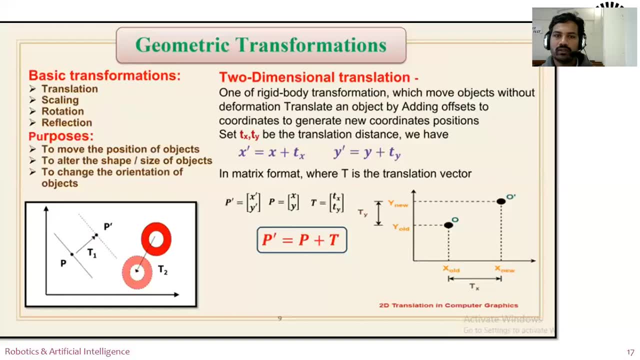 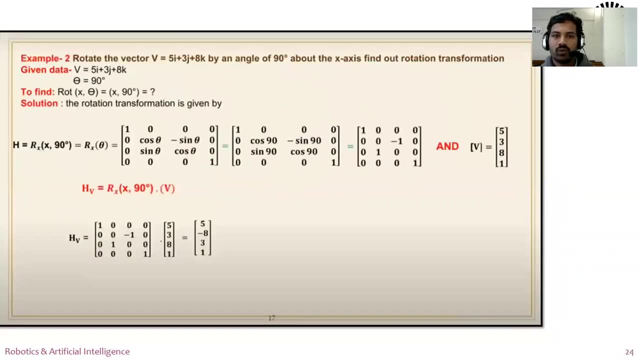 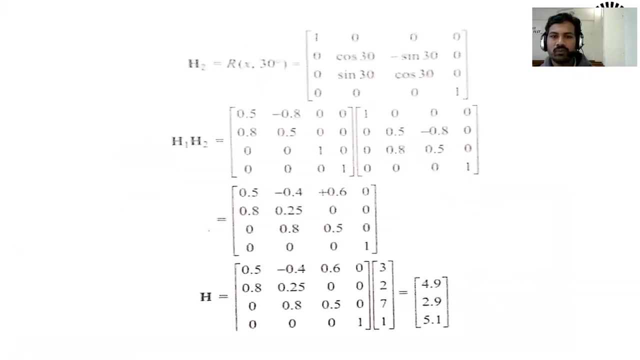 forward kinematics of three degrees of freedom robots. we have seen inverse kinematics of two degree of freedom robot. okay, geometric transformation we have seen. okay, this part also. we have seen in last lecture- homogeneous coordinates problems. we have seen on that. okay, these are the problems. again, it is uh, which is the previous we. 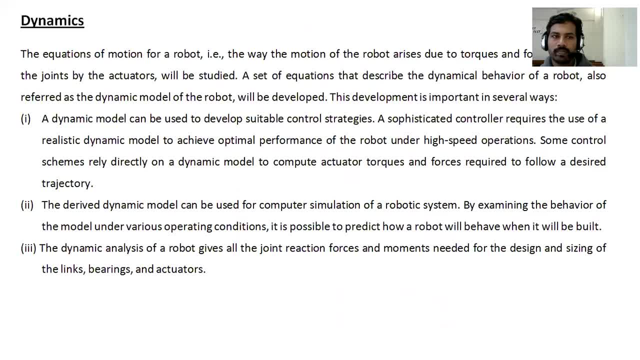 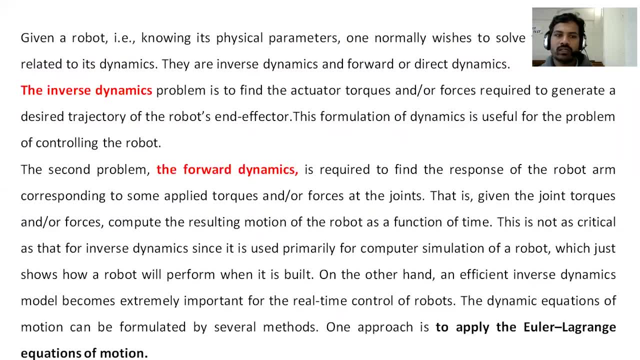 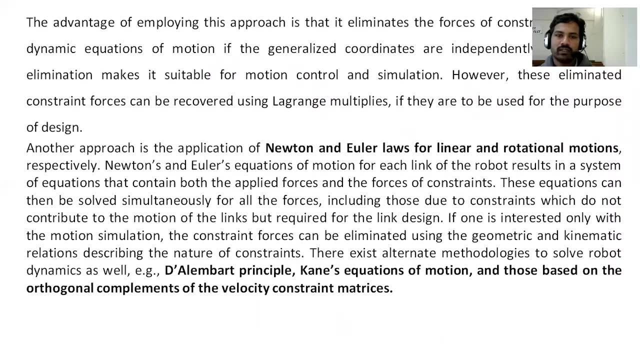 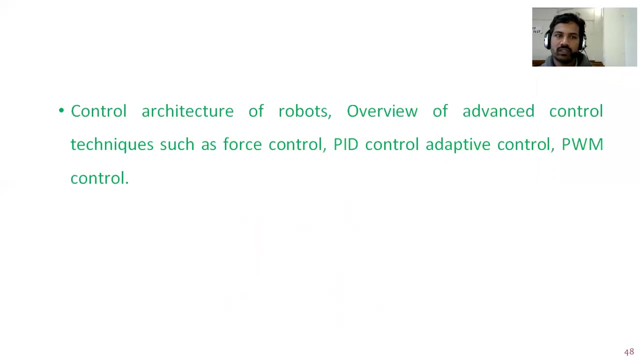 have seen that one. okay, i have just copied from book. the next, uh dynamics. uh, dynamics we have seen relating to, okay, inverse dynamics and forward dynamic. forward dynamics internalize the personal levels. dynamics, again, we have seen the robot arm dynamics. okay, this already part we have covered. next, control architecture of robot. in that linear controls, we have seen control techniques. 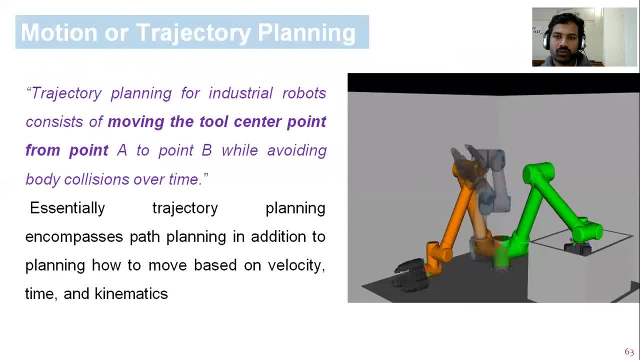 okay, like pid joint controller force controller- this already we have seen. now function emerged of your robot konuşے force controller. this already we have seen. now we are moving towards this motion or trajectory planning. okay, in motion or trajectory planning, in what we are, we are doing, we are just finding the. 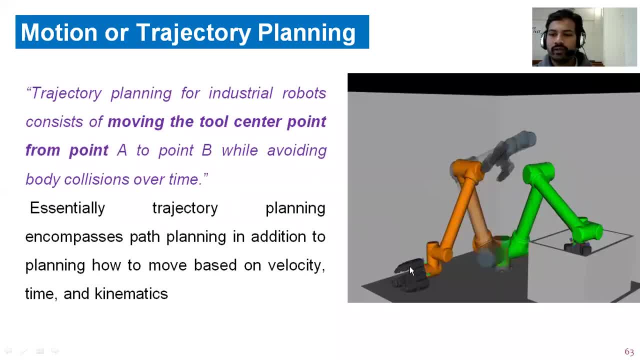 path of from start to end. okay, we are finding the path of the robot from start to end. okay, suppose here you can see in this animation from green color, the robot will start and end with this. okay, position means this motion or the path followed by this robot. it is nothing but our. 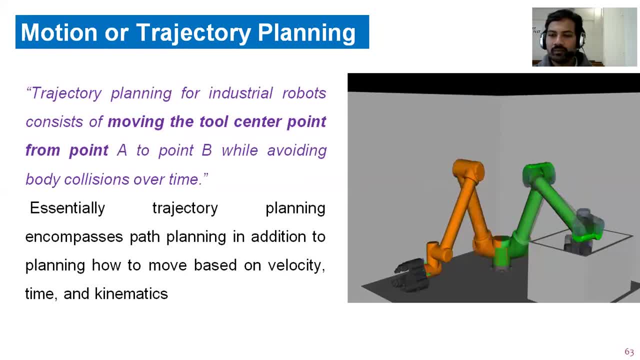 motion or trajectory planning means. what it means is very simple. language says: this is what you think. this robot, from the starting point to the end point, the path followed by this robot, is called the trajectory of that robot or motion of that robot. okay, here also that one I have written. trajectory planning for industrial robot consists of moving. 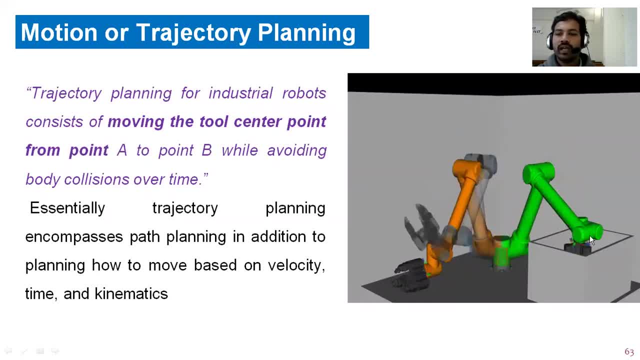 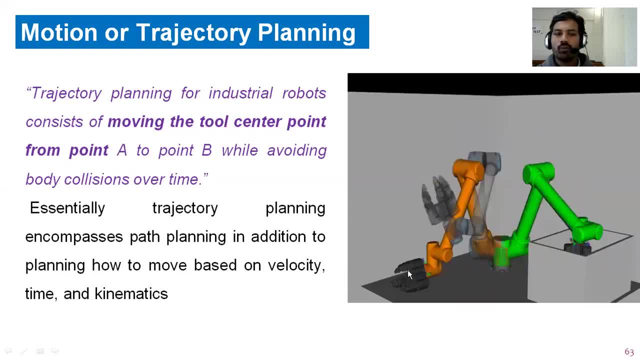 mood point: is B okay while avoiding body collisions all time. okay means what it means: is that body okay when we move from A to B? then in that, any fluctuation in that link of the robot, there is no complication in that movement okay over time. essentially, trajectory planning encompasses path planning in addition to 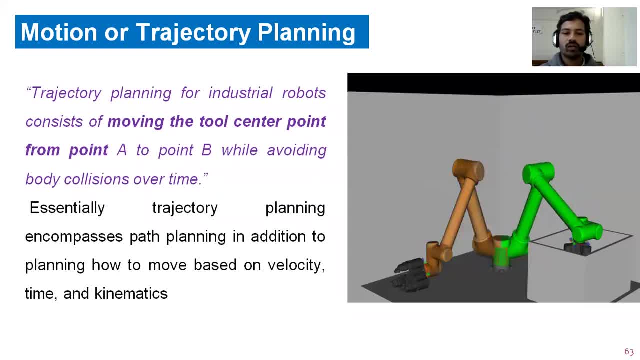 planning how to move based on velocity, time and kinematics- okay, this in trajectory planning. we are going to study path of robot. okay, path of robot which is based on velocity, time and the kinematics- velocity and time and kinematics- with the lapentatikani discuss kind of okay now there. 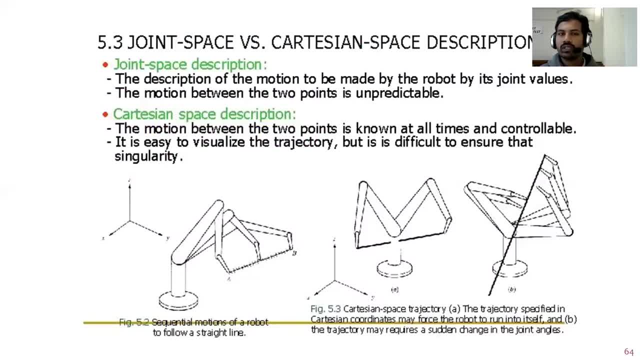 are two methods of this trajectory planning. which are those? first one is the joint space and the second one is the trajectory planning. okay, now there are two methods of this trajectory and the second one is the cartesian space. okay, two methods are there in this method. first is joint space trajectory planning and second one is the cartesian space trajectory. 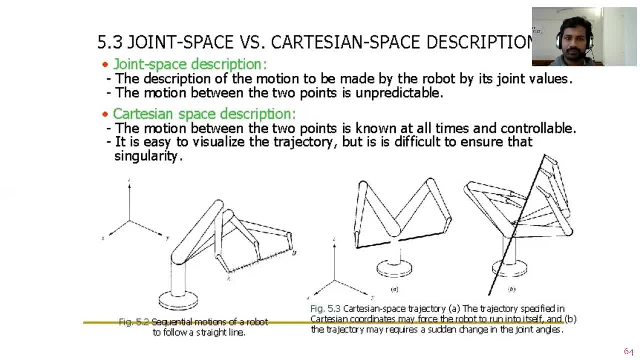 planning in joint space description. okay, what is mean by joint space? now we will discuss. okay, what is joint space and cartesian space trajectory planning, What we do in trajectory planning, Let's study it first. Okay, You can see, in joint space trajectory planning we are dealing with motion of the robot made by the motion of the robot, made by the robot by its joint values. 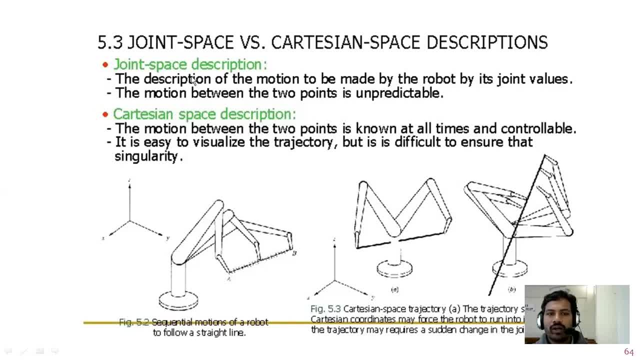 Okay, Once again I will repeat: in the joint space trajectory planning, we are dealing with motion of a robot made of robot by its joint values. Okay, In the joint space trajectory planning, we are dealing with motion of the robot by its joint values. 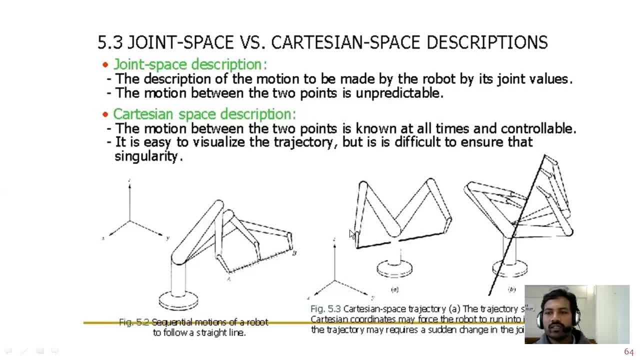 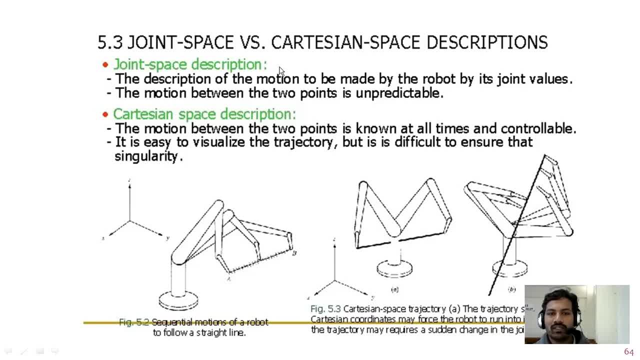 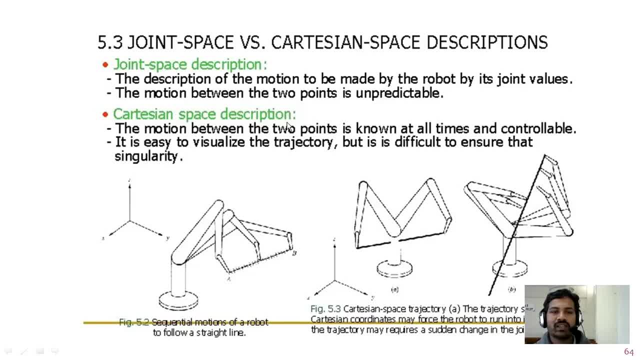 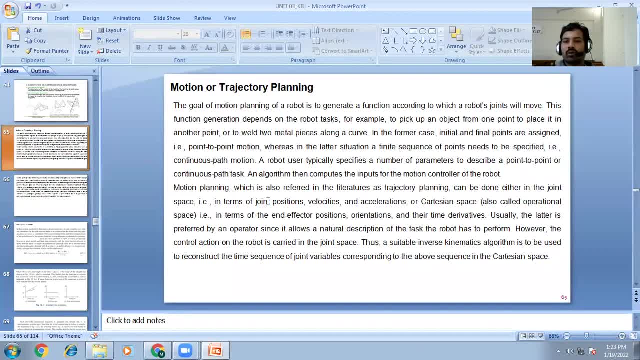 it depend upon the operation performed by that robot. okay, now suppose we have the robot pick and place, as in that case, we just pick up that object from one place and we are placing to the another. okay, or suppose one welding robot is there. okay, welding is a robot, as in that case. 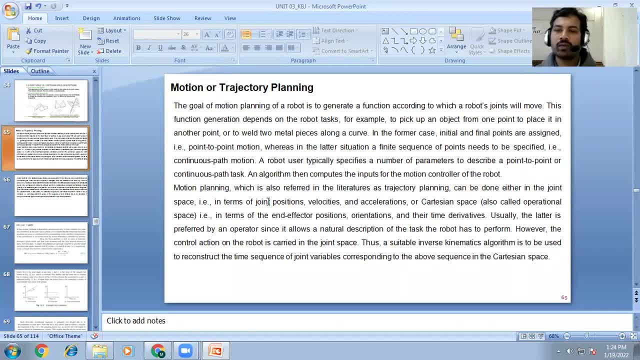 we have to weld. suppose a car body you are going to weld, then that car body is not in a straight line. okay, here that robot motion must be in a curved manner. in that case we have to use this trajectory planning or we have to define the path of that end effector. end effector. 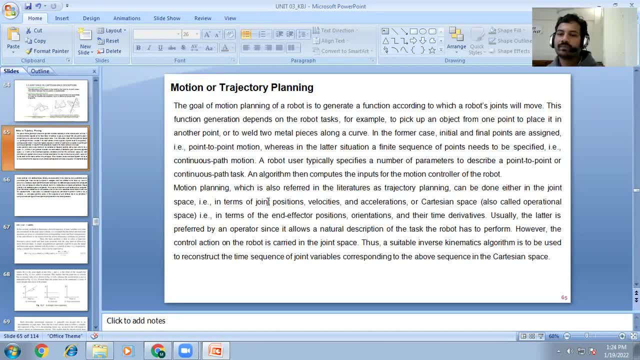 path that you can define. in the former cases, initial and final points are assigned, that is, point to point motion, where in the latter situation of finite sequences of points, you can define the path of the robot in a straight line. okay, here that robot motion must be in a. 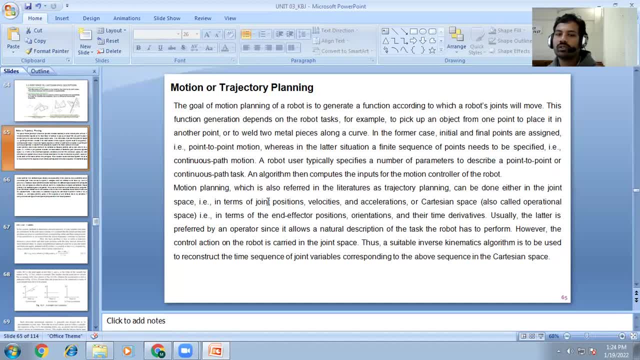 need to be specified, that is, continuous path motion. a robot user typically specifies a number of parameters to describe a point to point or continuous path motion. okay, sometimes we required to move the robot point to point or sometimes we have to require to move the continuous part point to point where we can use pick and place robot where required. point to point motion. 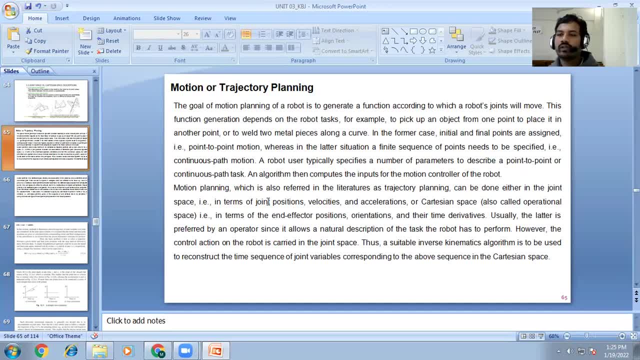 and in welding we required a continuous path motion. okay, to measure, bag it- Lhasa's the peak- and place as a robot a center tab to Kenny we have to use for a point-to-point motion and in welding operation we have to use the continuous path motion robots. okay. 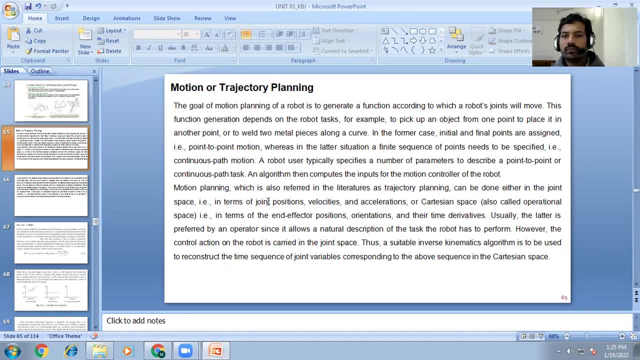 next one is the robot user, a typically specify number of parameters to describe point to point motion, point or continuous part task. an algorithm then computes the input from the motion controller of the robot. motion planning, which is also referred in literature as a trajectory planning, can be done either in the joint space, that is, in term of joint position, velocities, acceleration. 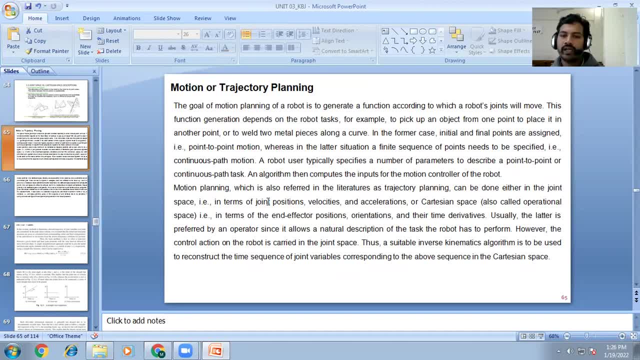 cartesian space, that is, in term of end effective position orientations, their time derivation. usually the later is preferred by an operator since it allow a neutral, natural description of the task that robot has to perform. however, the control action on the robot is carried in the joint space. the suitable inverse kinematics algorithm is to be used to reconstruct the time. 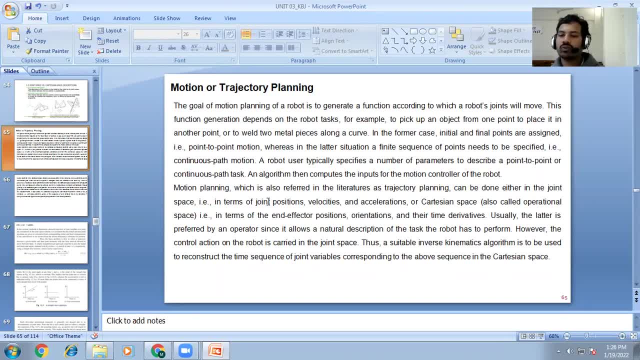 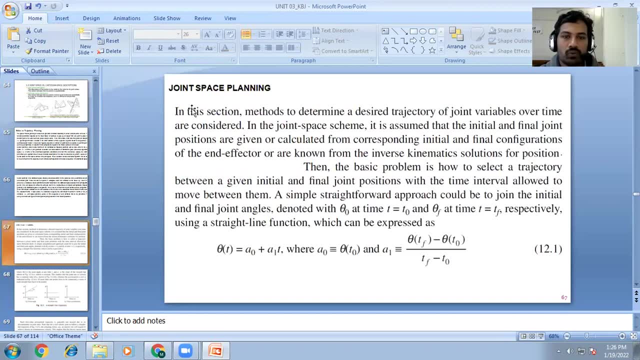 sequence of joint variables corresponding to the above sequence in the cartesian space. okay, next one is the first one is the joint space plan. the joint space plan- just before that we will see one video related to joint space and the cartesian space. means we can understood that. okay, joint space and cartesian. just. 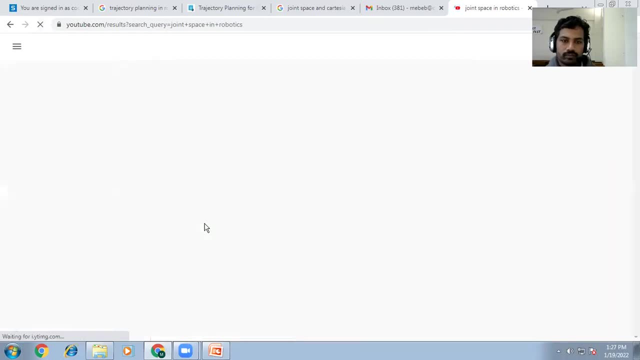 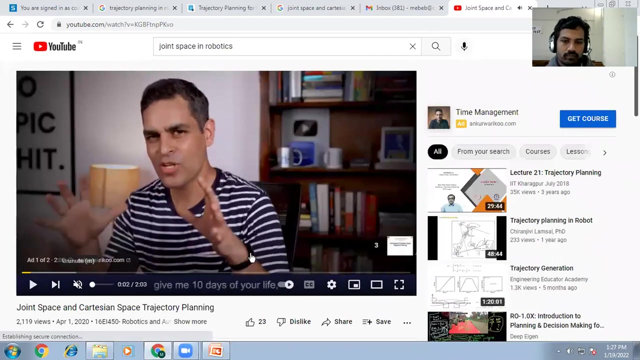 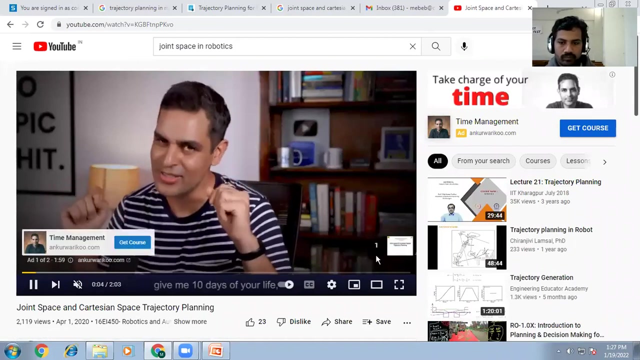 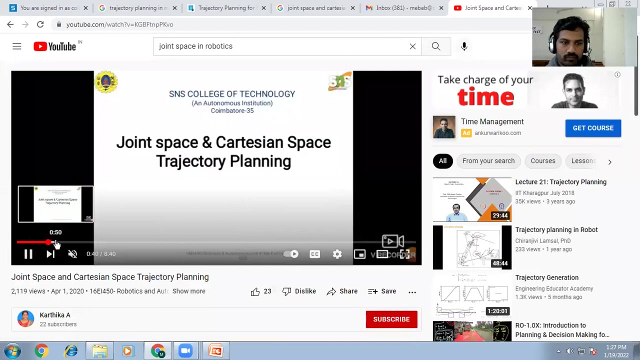 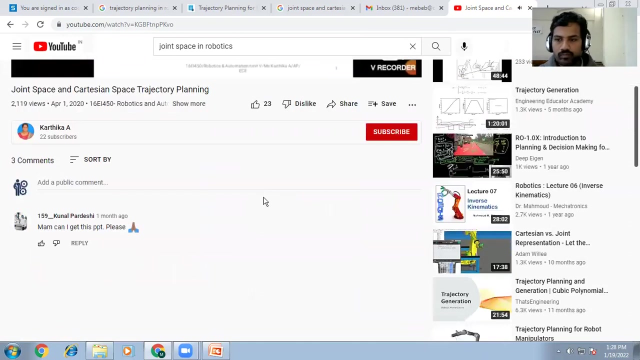 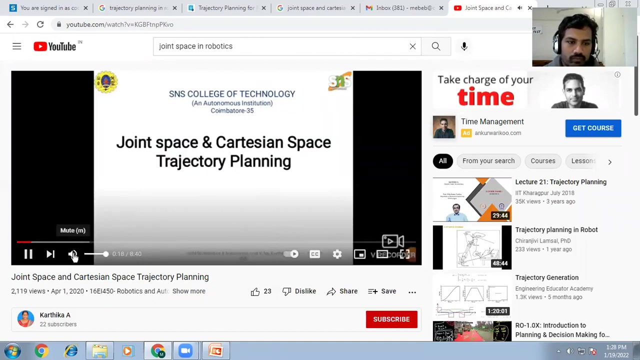 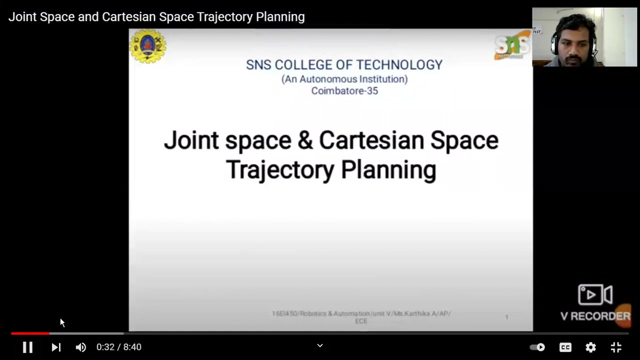 before that we can understood that the the The goal of trajectory plan is to distinguish between the two, namely the path of the project, the path of the control, the mean, the immediate path of the project and the derivative path. These are generated by interacting with or approximating the business path by a polynomial. 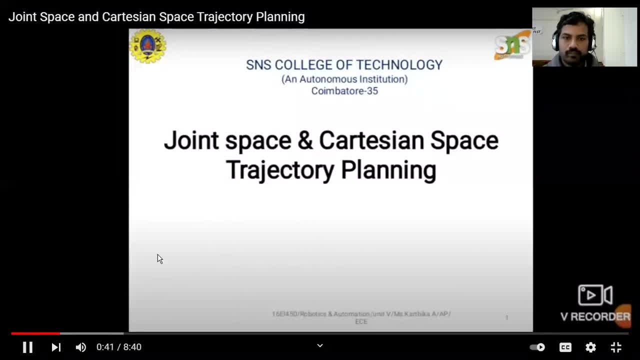 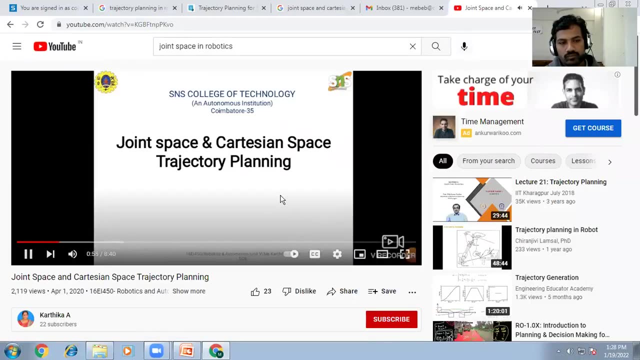 function. So what are the terminologies in trajectory plan, In this data path trajectory knot points arc via. points are interpolation points. First one is path. A path is the notice of points which travel through the magnetic field of the expected. 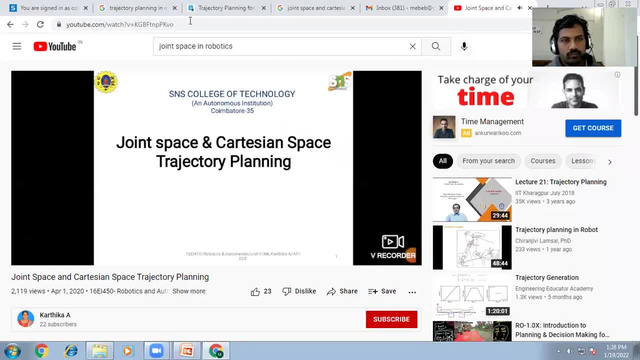 vector Trajectory. A trajectory is a path in which a particular direction is a path and its time is specified in terms of velocity and acceleration at each point. In particular, a trajectory is the time sequence of the trajectory, Velocity and acceleration for each join or change vector at the magnetic field. 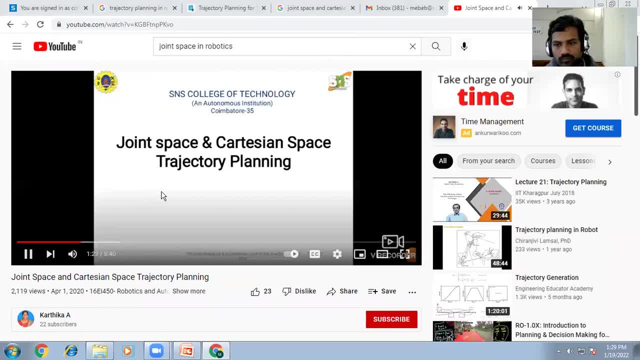 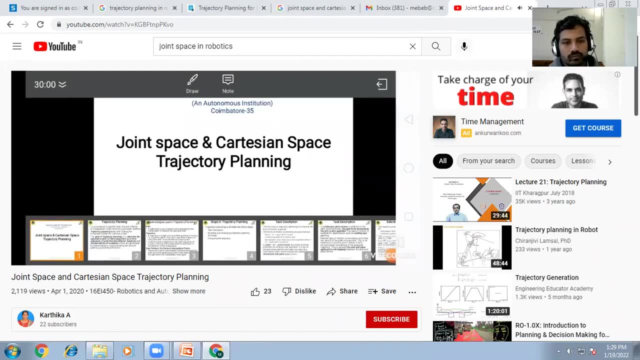 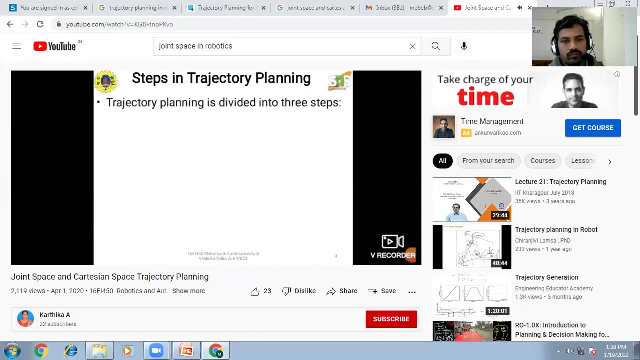 Knot points or minor points are interpolation points. These are the set of preconditions between the start points, destination points, on the trajectory in which the manipulator knot paths. Next let's see trajectory plan. First one is path. A path is the position of the trajectory when the possibly target point is pointed. 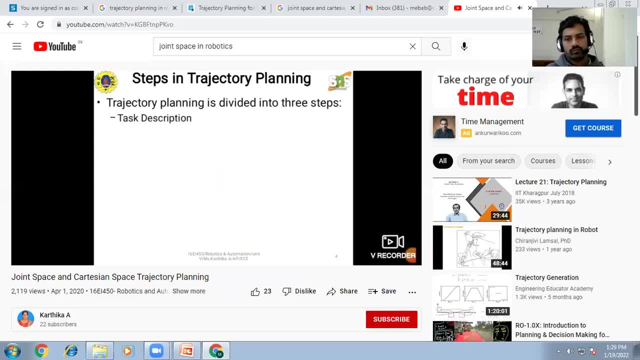 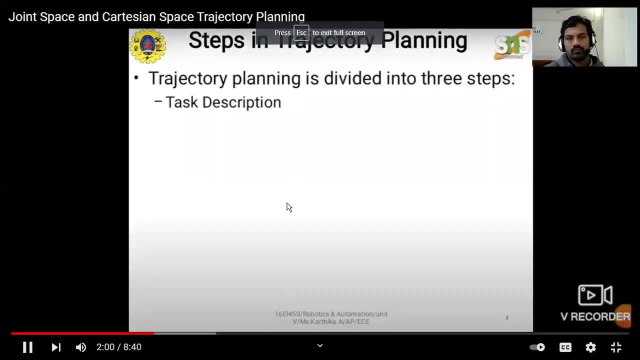 in the direction of the orbit. In the third one is path. A path is the position of the trajectory when the possible trajectory point ends in the direction of the orbit. In the fourth one is path. In the sixth one, the trajectory is the time sequence. 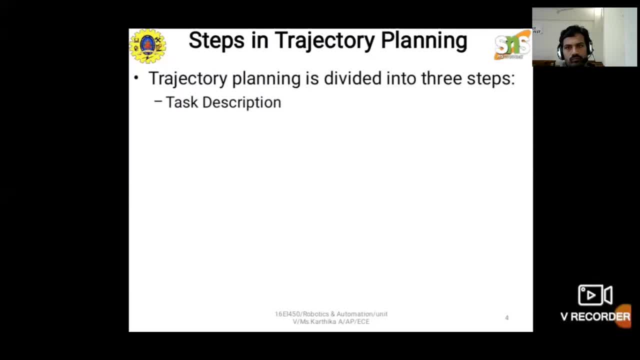 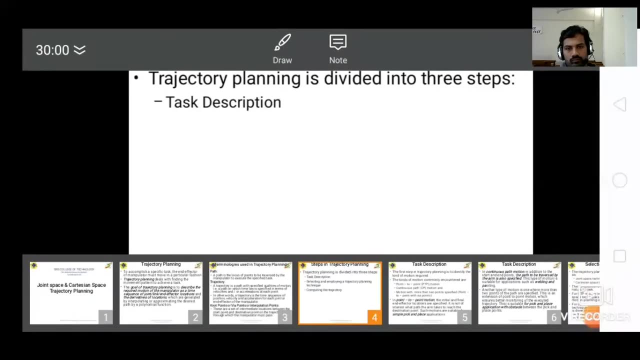 point-to-point P2P motion, continuous path motion, CT and motion with label 2.65,. point-to-point with y-axis. So what is point-to-point motion? It is the actual indicator location for a specific path, So you have to be sure what the path is. 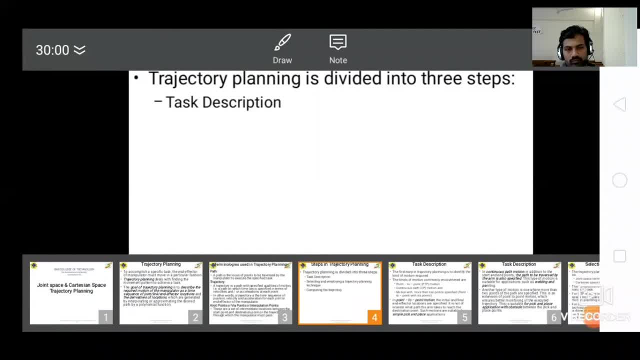 So this is the point-to-point. So this is the point-to-point. Next one: continuous path motion. in addition to path-based motion, the path to be traveled is almost always specified. This type of motion is suitable for applications of P2P motion. 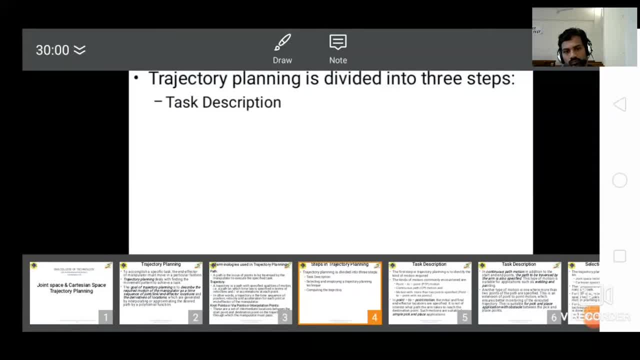 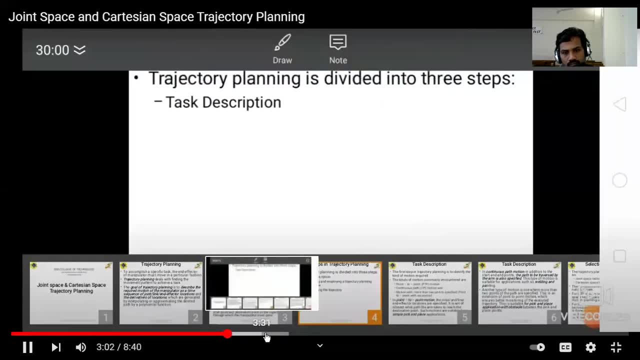 I will talk about why that mobile P2P is specified. P2P is a series of point-to-point motion which ensures better mobility of the educated path. So you see that the P2P motion is more stable than the P2P motion. 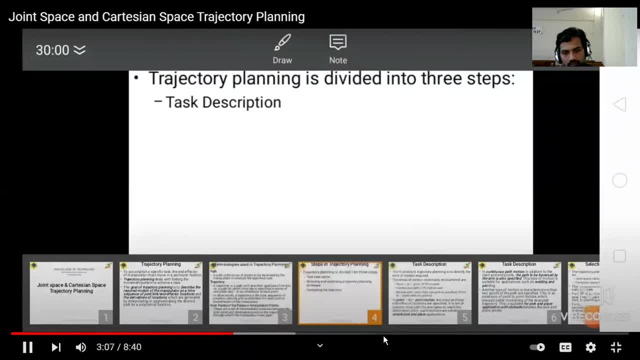 So this type of orientation of the P2P motion is employed for the pose movement and for the transition. So the P2P motion is displayed at the P2P Во educational center, And P2P motion is displayed just a fewdle different ways than the full census P2P motion. 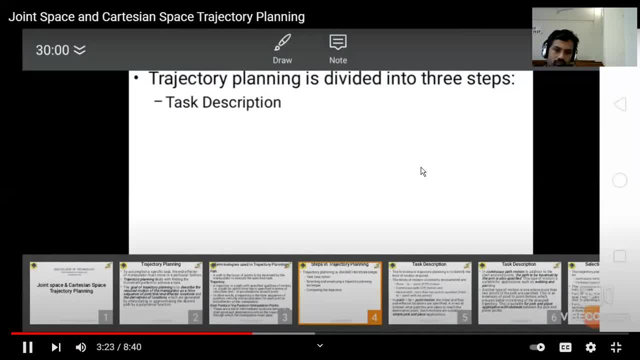 For the p2P motion. the third part-triangle method is different from P2P method. for P2P motion, P2P motion is the function of P2P motion, that is, the moves feed, a limit of one or theround speed of preparation. 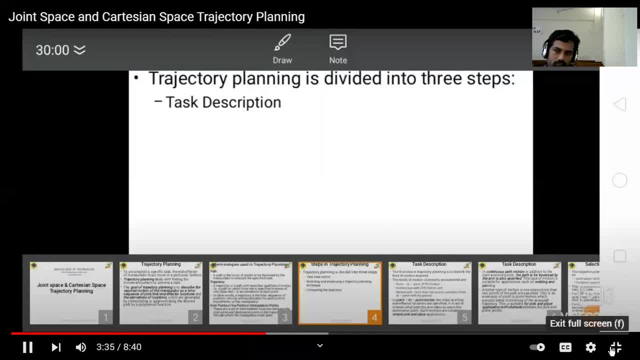 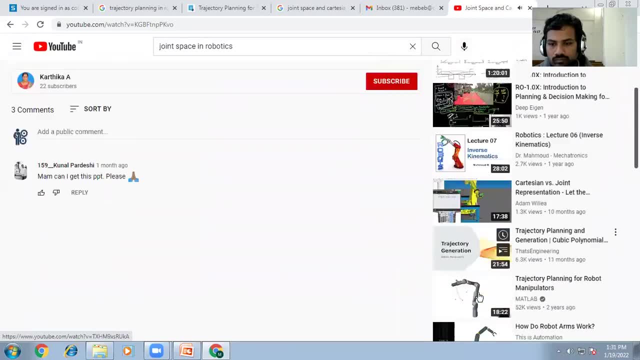 The rulesuyu p2p motion have different parameters. start motion causes you to take a side move, while the motion planning is direct in the pattern of the move. In this case, the join variables require to achieve a clear in the pattern of the move, while the system 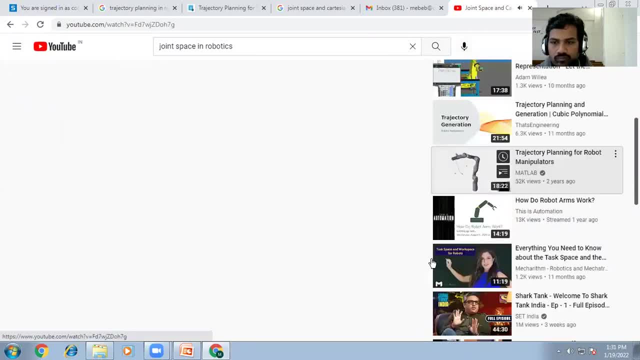 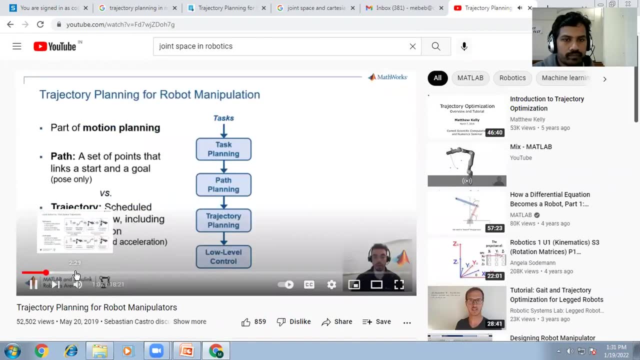 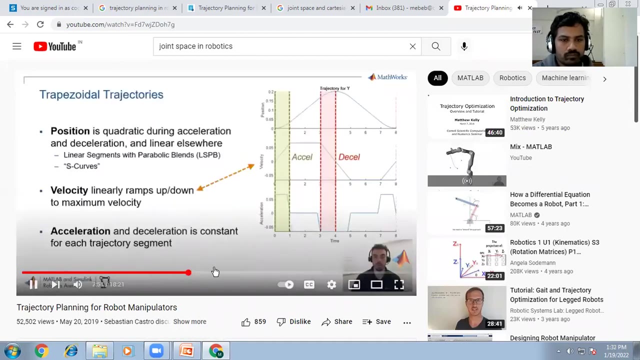 is in its way. Hello and welcome to the MAT11 simulation. It's a set of points that will link between a start and the goal pose, for example, whereas the trajectory that with the task-based trajectory some redundant, will be applicable to the model's lens. 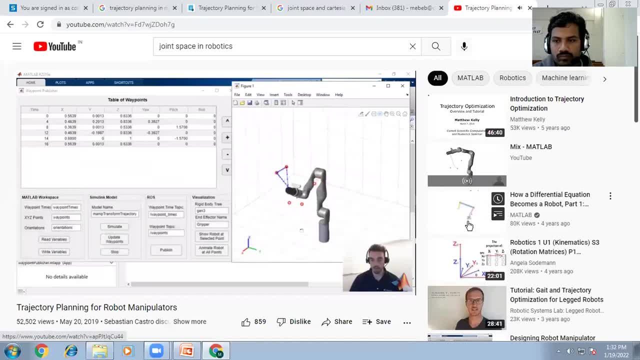 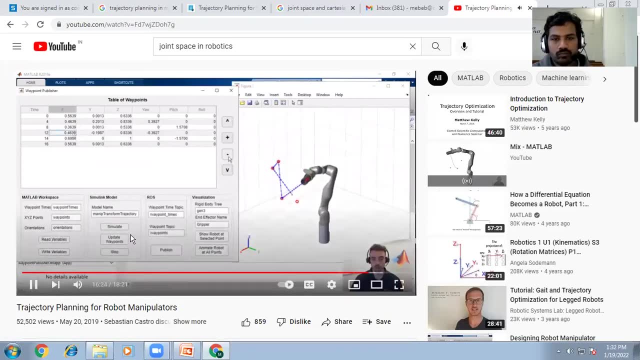 Then now you'll see that the following problem is a little bit different and our robot is now going to this last waypoint that we introduced up here, And then I can always, you know, also remove waypoints, republish and then see how that changes. 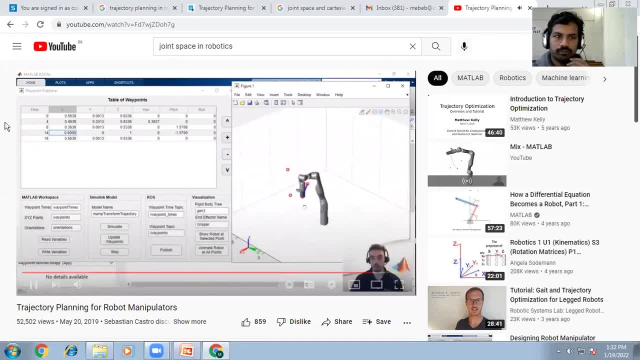 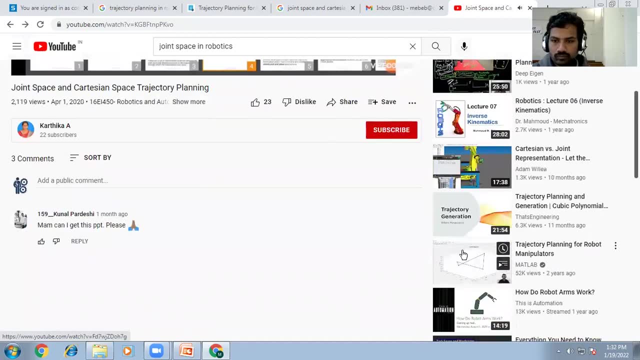 So obviously, and right now we have a MAT11 app talking to the simulink- but Next, how to compute a new trajectory. The final step in trajectory planning is to compute the time period of value at which the response can be set from the trajectory planning. 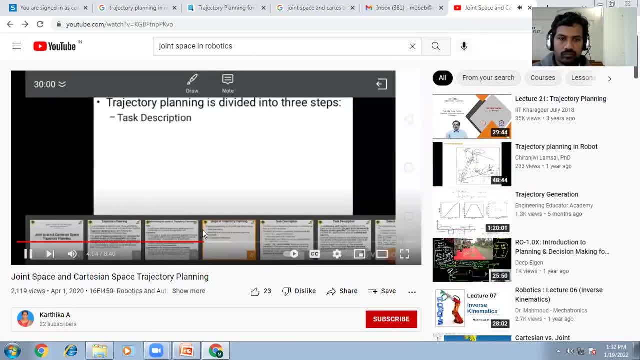 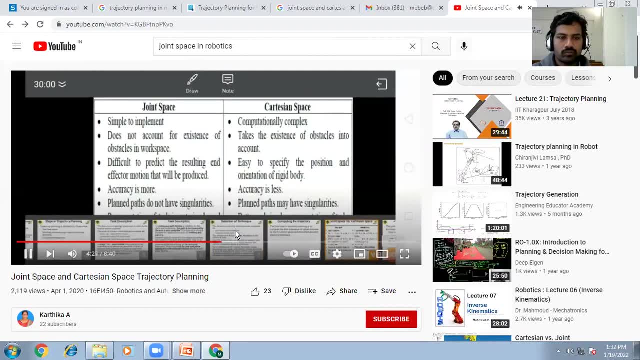 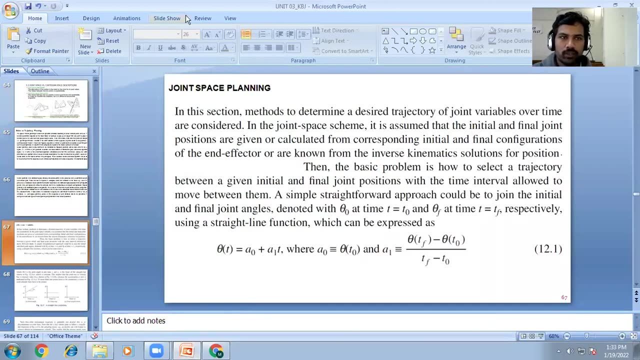 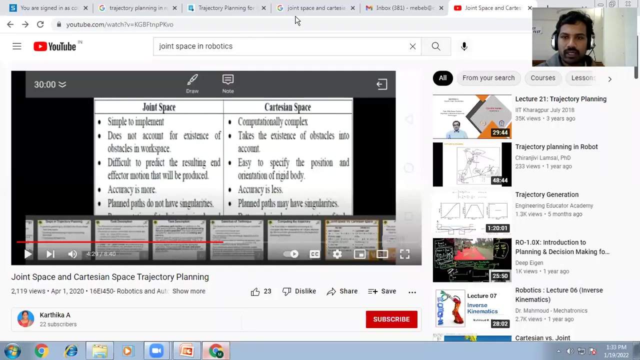 We actually need to have two methods. First, join state, particular partition space. What's the difference between dot and partition space? OK, You go through it. Actually there is no specific. you can say that the video, it is related to that- joint space and partition. 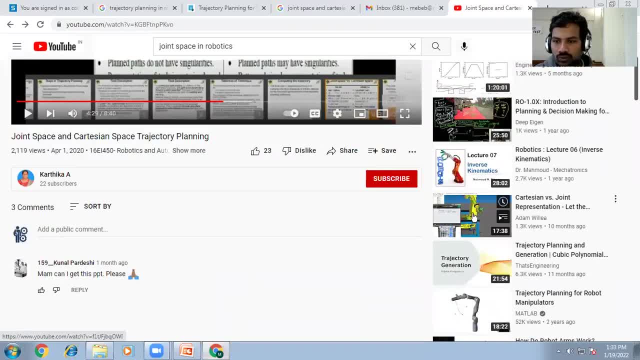 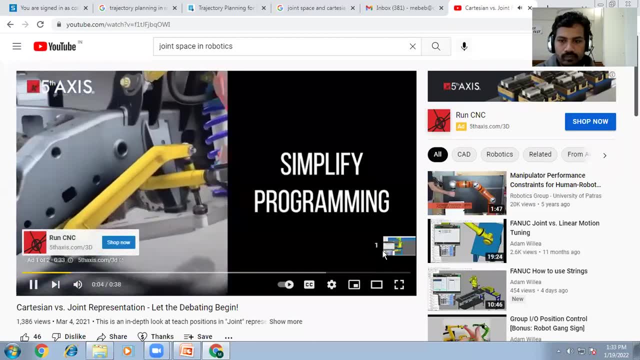 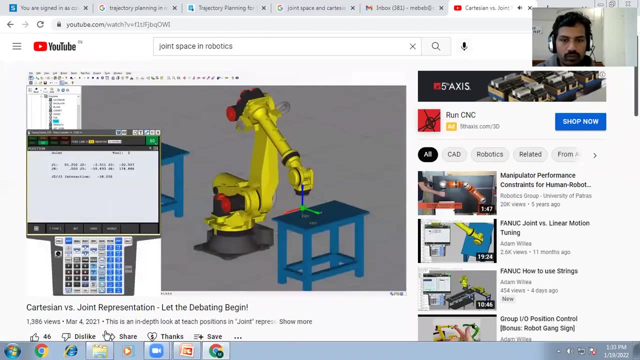 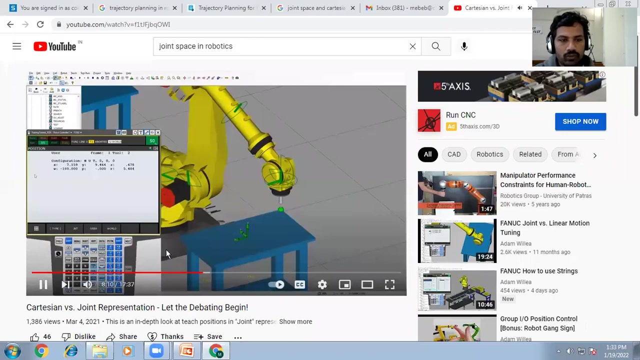 Just I want to observe you how exactly that robots are — With the RackLock QuickChange system from Vip Access, you can simplify your program. OK, Hey guys, Adam, these are advantages to centerline objectives before SLA. Here you can find the joint representation: 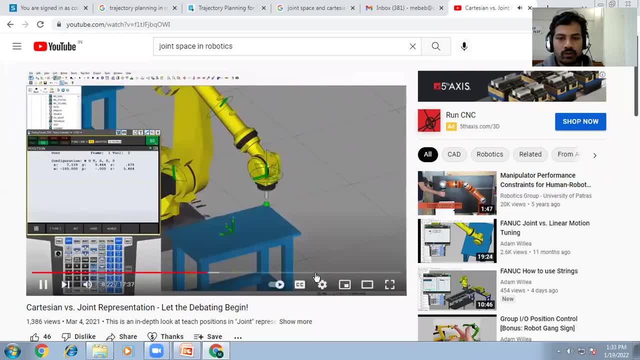 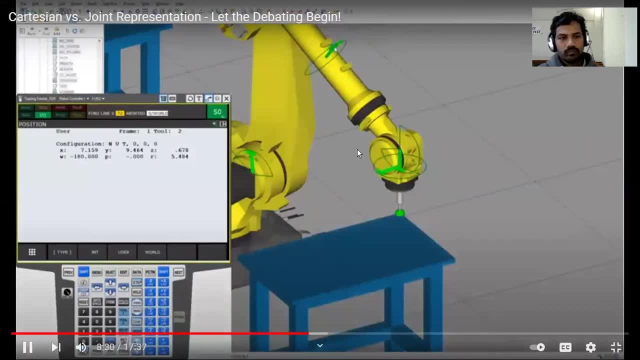 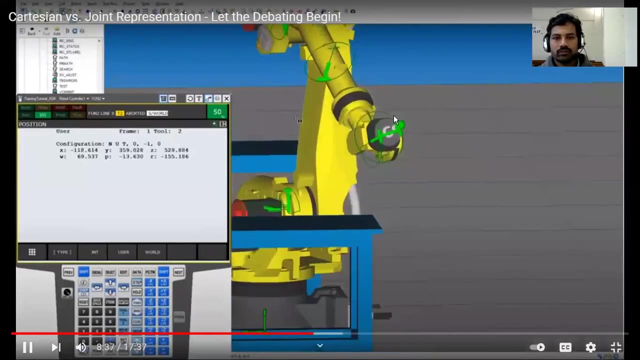 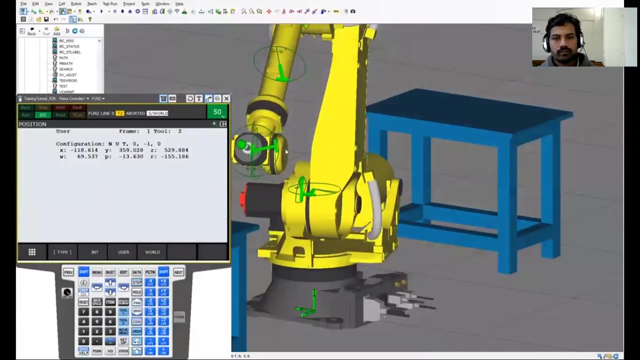 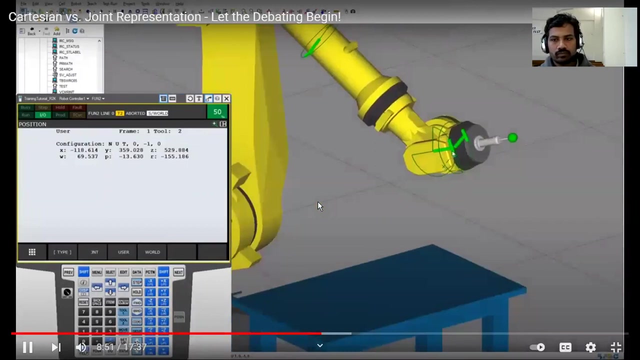 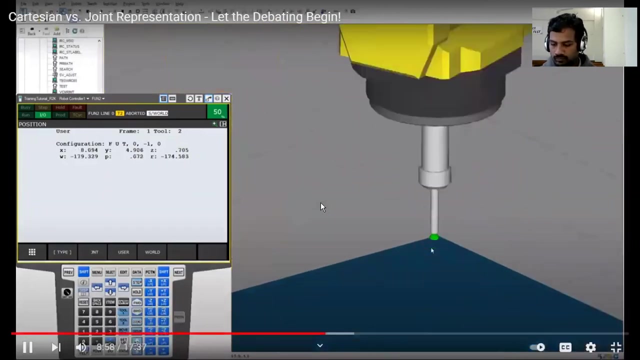 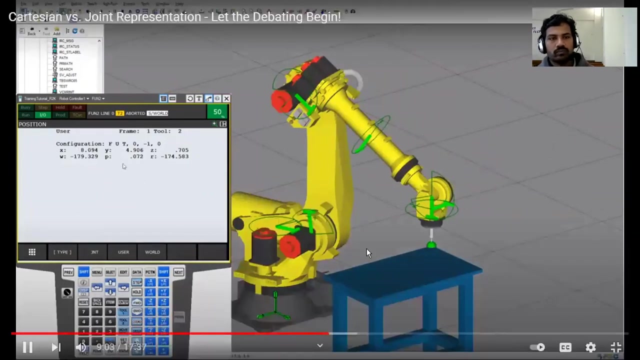 This robot right now. I have it. You can see here, You will understand. This one is the joint space Right back exactly where I began. Look at the difference. Yeah, Instead of the end, UT meaning not the end. 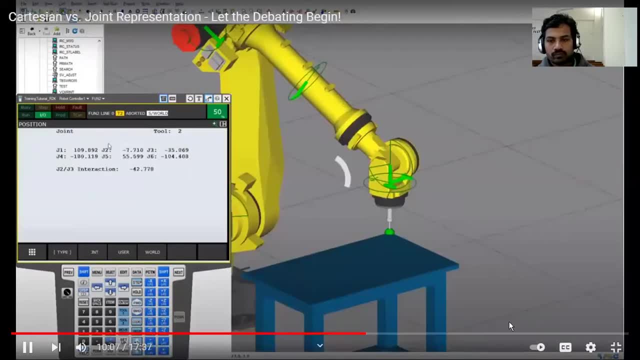 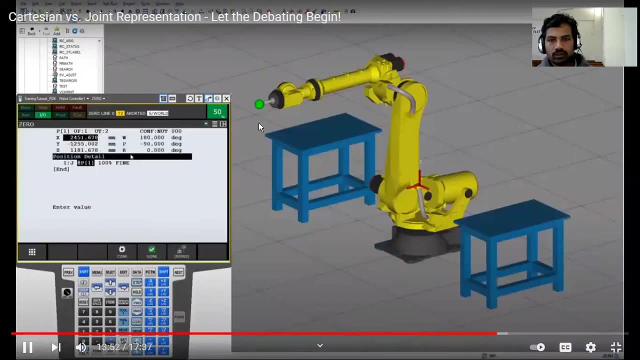 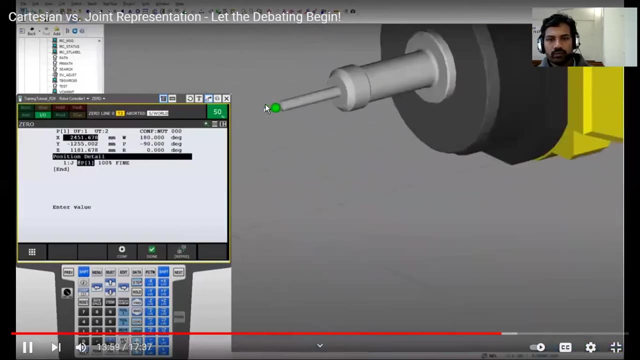 centerline bar or drop. That's because Why would I look at this thing as a fusion? These are the connotations with respect to base. This position is calculated The end of. At that point they have shown There is the base of the robot. 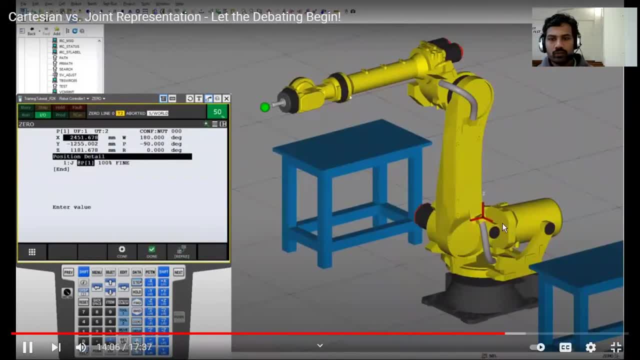 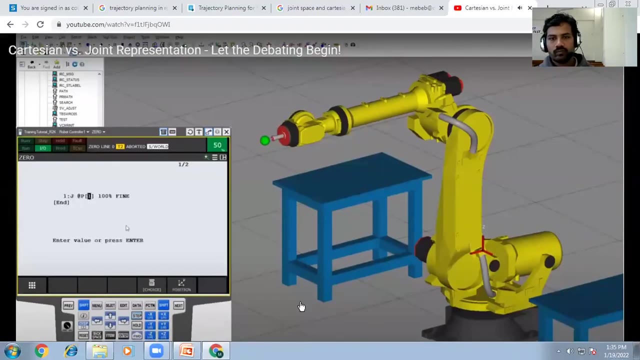 Okay, Here you can see also. Here also it is written with respect to this base in Cartesian coordinates. Another question: This should be your first power-up question: Do I need to use a joint condition to go to a joint position? Okay, 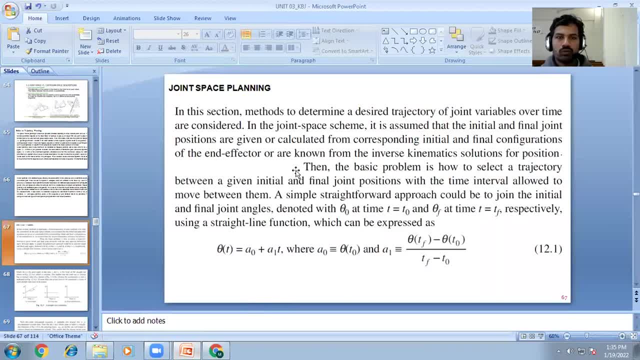 Let it be, This is Yeah, I want to just show how to do that, The joint space and the. Just remember that if, with respect to joints, The In Cartesian, just we are doing in the form of coordinates, Okay, 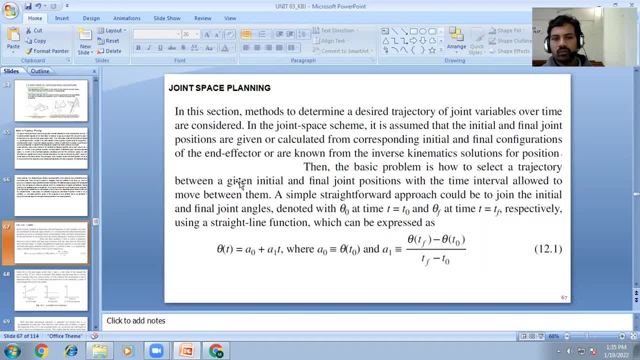 Jackal coordinates along X, Y and Z, The motion or the path If you want to find, then in that case we can go for the Cartesian space and in joint space, in joint space, the depend upon the angle in this section, method to determine. 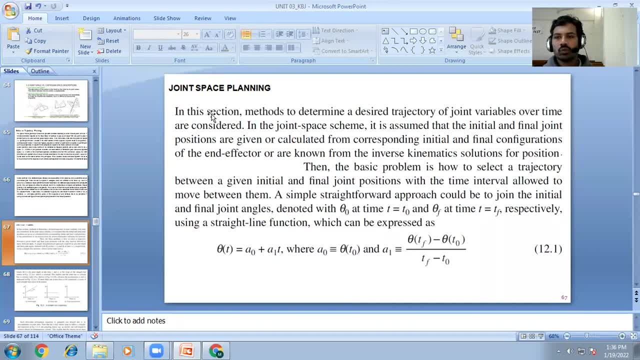 or describe trajectory of motion variables over time are considered in this joint space scheme. It is assumed that the initial and final joints position are given are given or calculated from corresponding initial and final configuration Okay Of the end effector, or are known for from the inverse kinematics solution for position. 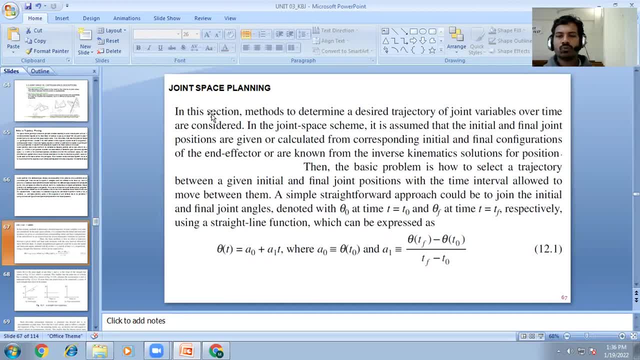 Okay, Joint space in that we are doing similar to inverse kinematics: at the inverse kinematics to find the position of end effector. Okay, To find the position of end effector, or the. simply we can say that if I know the position of end effector, 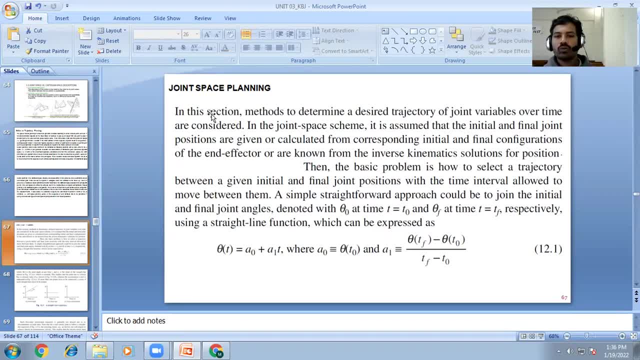 And from that we are finding the angles of each joint. protect joints. I find out similarly in joint space planning. Also, we are using the inverse kinematics to find the position of each angle. Okay, But take angle to position to find out the result of that case. 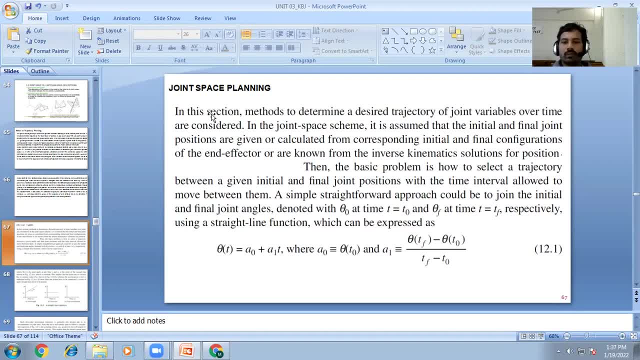 When they inverse kinematics use kind of. then the basic problem is how to select a trajectory between the angles. Then the basic problem is how to select a trajectory between the angles. Then the basic problem is how to select a trajectory between the angles When given initial and final joint position with the time interval allow the move between them. a simple 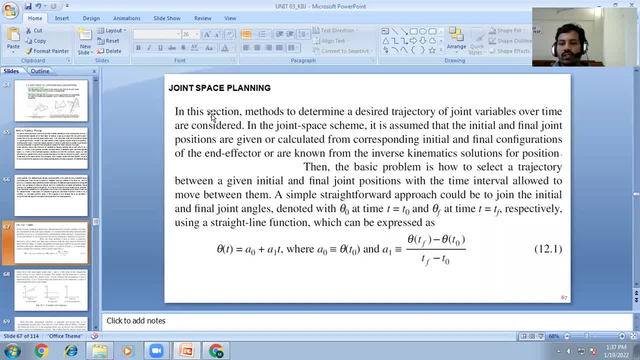 straightforward approach could be To join the initial and final joint angles denoted with theta 0 at time 0, theta f at time t f respectively, using straight line function which can be expressed as: Okay. how can you represent Why any straight line person: theta t is equal to a 0 plus a 1 t. 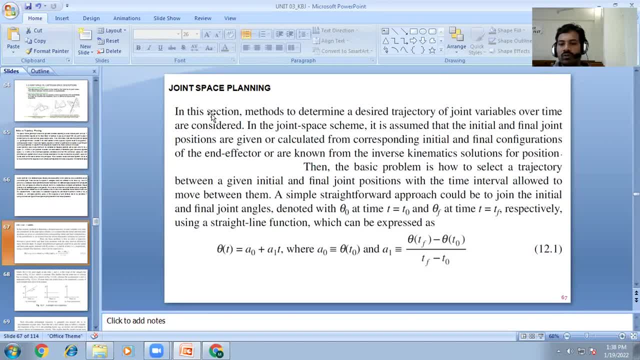 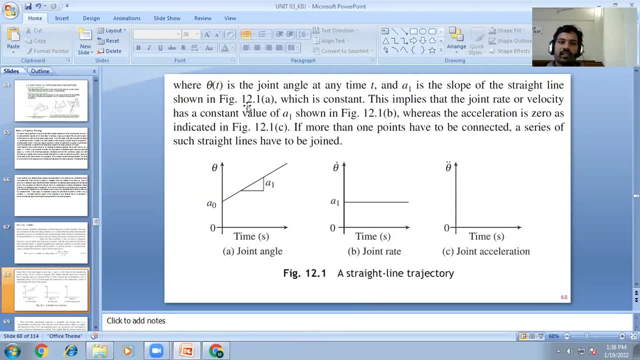 Okay, a 0 is theta t 0 and a 1 is the this angle value. The next one is the, where theta t is the joint angle at time. t and a 1 is the slope of the straight line shown in figure, which is constant. 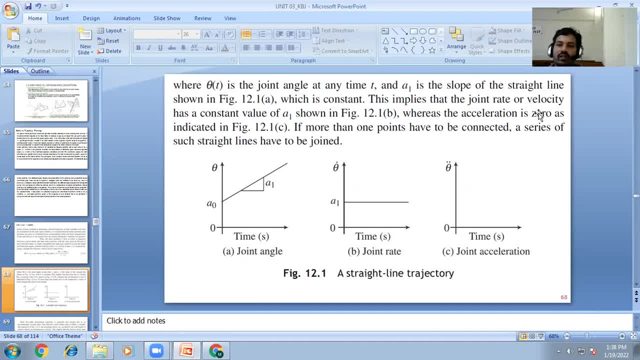 This implies The joint rate, or velocity, has constant value of a 1 shown Where acceleration is 0, as in Indicated in finger. you can see it here. Here you can the join to rate at the joint angle with respect to the time. 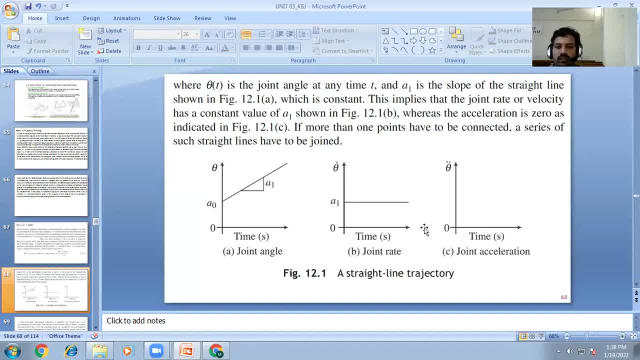 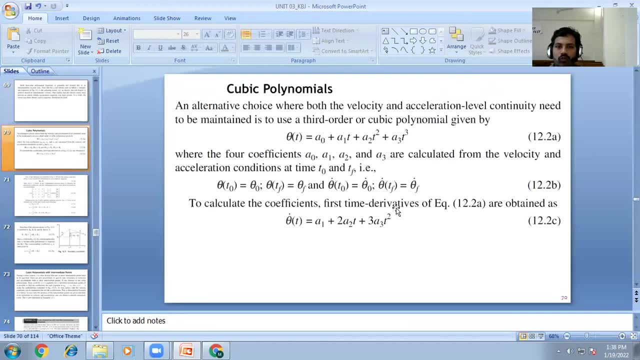 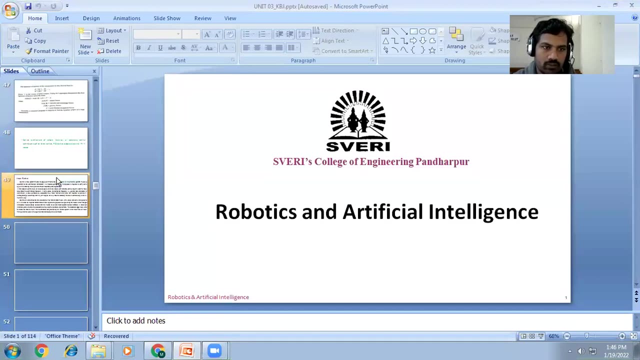 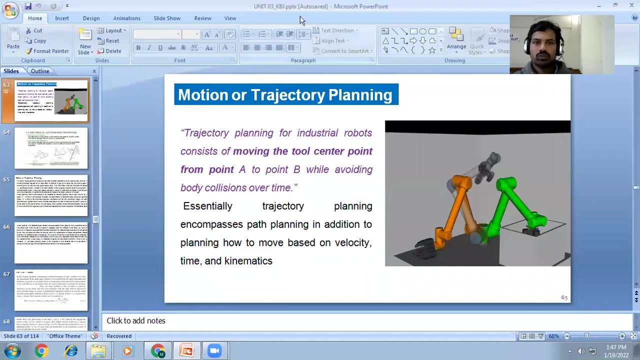 If it is changing the slope. they have shown, OK, Joint rate and joint acceleration slope. they have shown you, Nick. okay, we have started our trajectory planning. where we are, just i will go fast. okay, we have seen what is mean by motion of the trajectory planning. 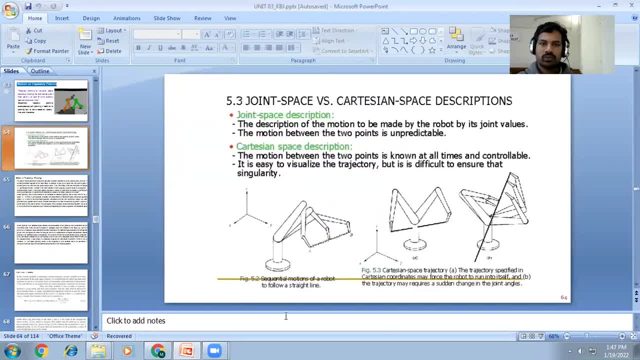 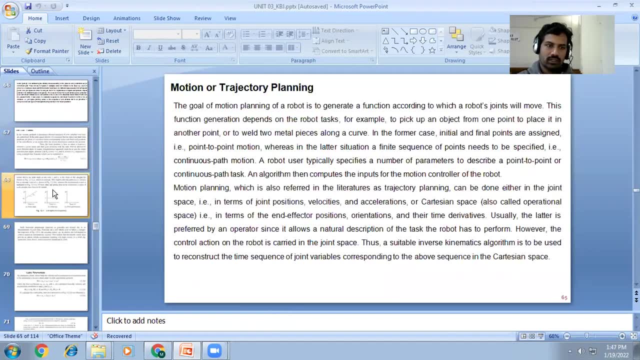 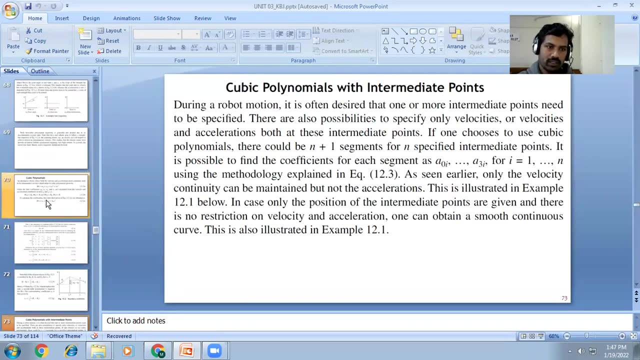 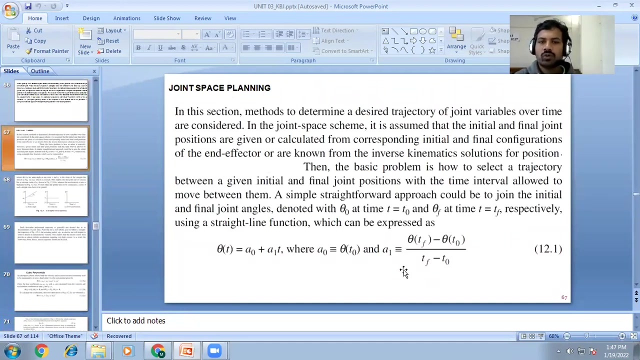 okay, after that we have started. we have seen the joint space and cartesian space. after that we have seen some of the related to that trajectory planning. okay, next first one is that in that we have seen the joint space planning for the. suppose you you want to move the robot in a straight line manner, then for that, 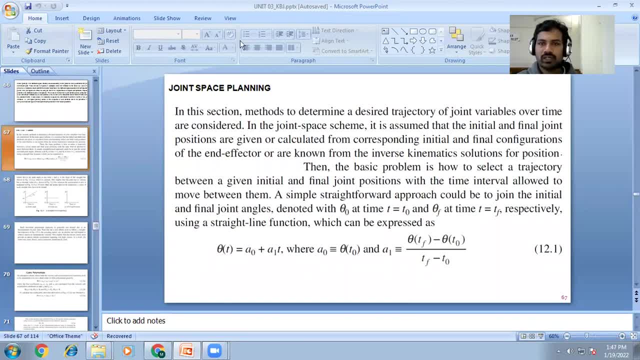 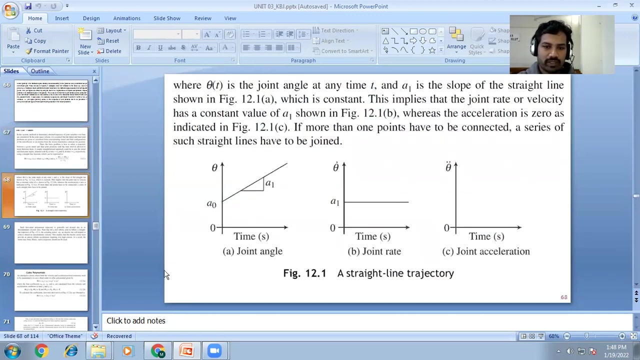 here that equation, it is a represent: okay, okay, simply, we can write: okay, suppose, okay, straight line. so the equation laser said that how we can write similar fashion. we can write for the: if you want to travel the robot in a straight line, okay, straight line manner. if you want to move that, in that case, if we can do something, we can write similar equations. 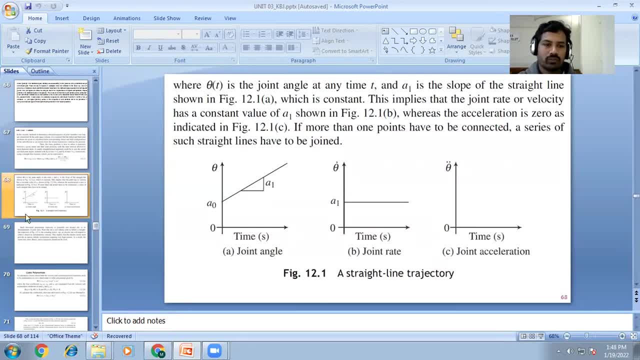 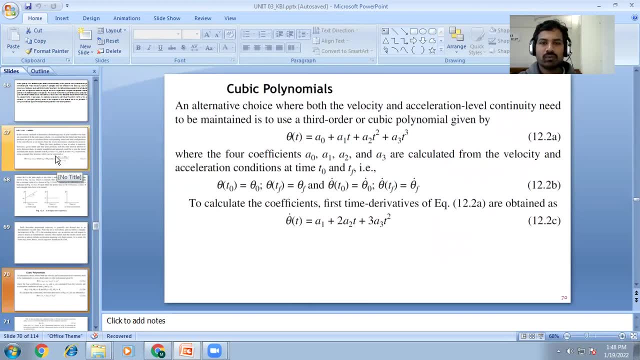 and depend upon the joint rate and joint acceleration we can write. next one is the. if it is cubic polynomial, okay. other straight line. straight line for that, now polynomial is not there. straight line for that, now polynomial is not there? a curve. Similarly, you require one cubic polynomial equation, like our theta. t is equal. 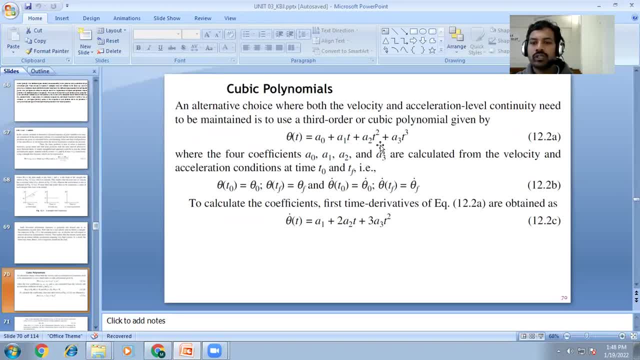 to a 0 plus a 1 t plus a 2 t square plus a 3 t cube. t is the time required. we can say that, and where we 4 coefficient a 0, a 1, a 2 and a 3 are calculated for the velocity. 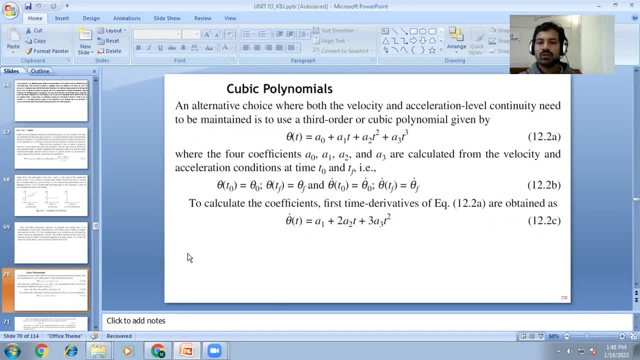 and the acceleration condition at time: t, 0, tf. that is initial condition time and final condition time. Ok, we can take the derivatives of that one and from that you can find out way to calculate coefficient. first time derivative are obtained as if I take the derivatives. 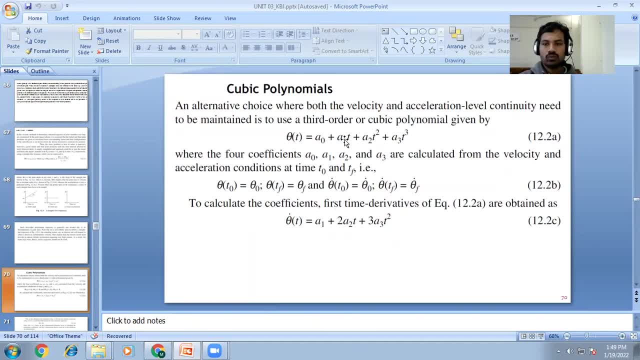 of t and t from t is equal to 1 t, 0 t cube. So we can write the acceleration and Tahitian the this equation 2, point 12.1 a. then the value we get. derivatives means we are finding the velocity of that joint. okay, the joint capital velocity. find out correct, okay. next, 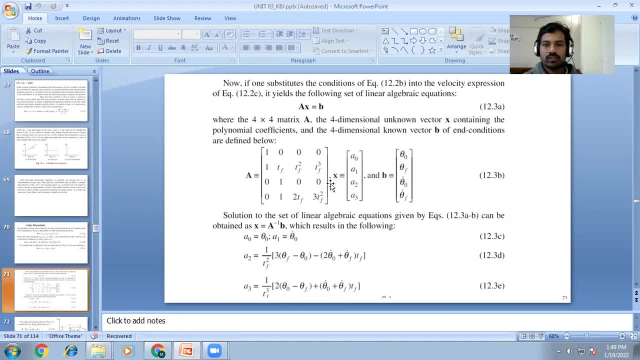 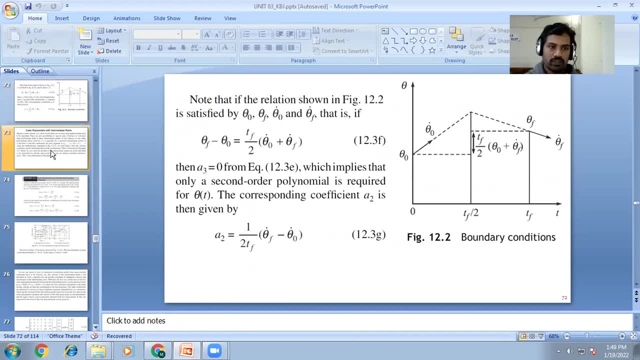 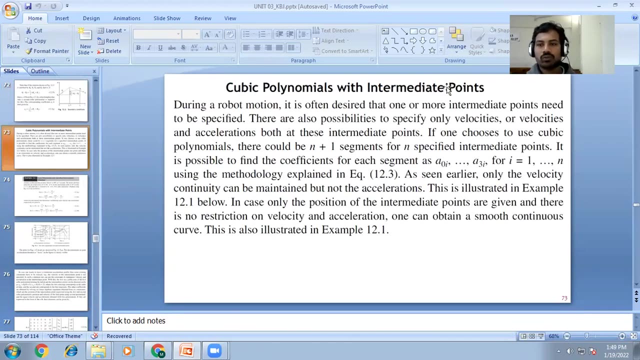 if i write in similarly matrix form, okay, linear algebraic equation, you will find such a format and from that you can find out the values. okay, cubic, polynomial and intermediate points: okay, suppose, if you want to find the intermediate points of that state space, okay, then in that case. 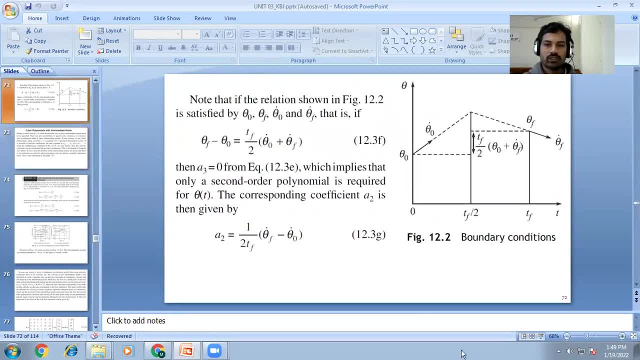 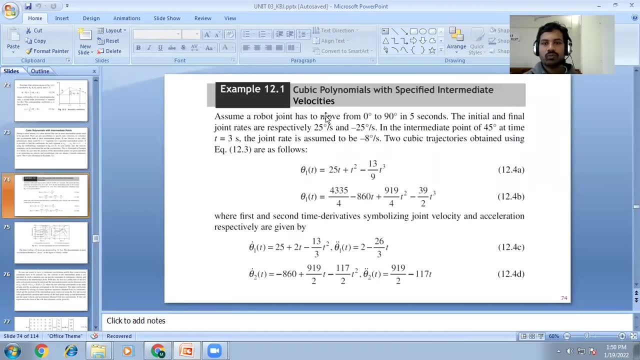 we can use such method- mathematical formulas- to find out. next, some of the example they have given. okay, example like cubic polynomial with specified you intermediate velocity. actually this is not part uh. they have not mentioned to test. solve the problems on this uh, cartesian and space test. okay, 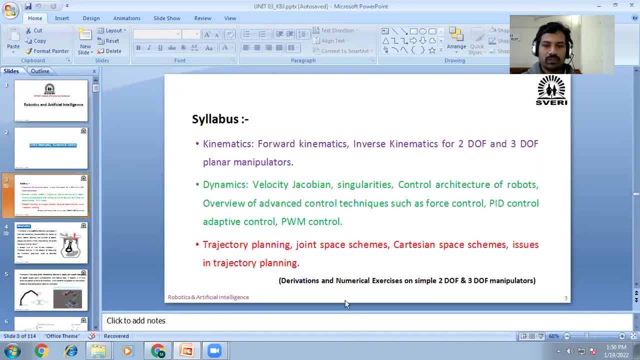 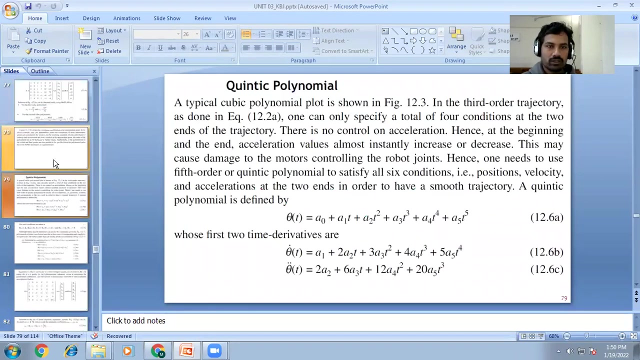 if you see your syllabus, okay, syllabus: derivation: numerical exercise on two degree of freedom and three degree of freedom. a manipulator means it is related to only forward and inverse kinematics. then also, just, we will take the one problem, a problem, how actually it is, find out with the help of this joint space where it is okay. this one is: 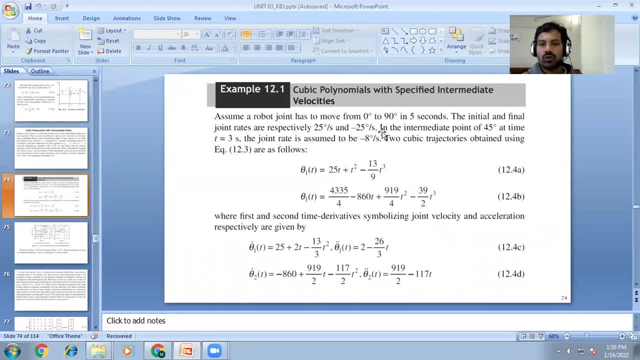 the problem. assume a robot joint has a move from initial condition they have given zero degree and at last condition is the 90 degree in five seconds. here to travel from 0 to 90 degree we required five seconds. for that they have given the and depend upon that. we have to solve the problem. 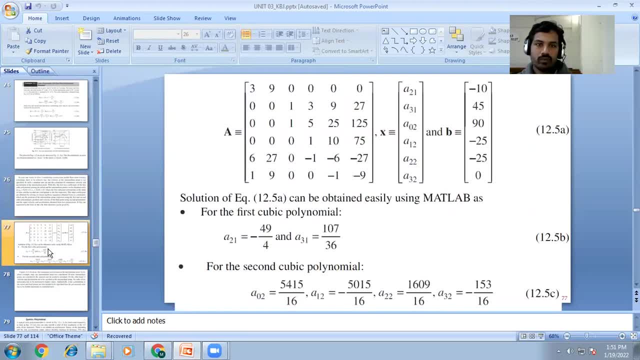 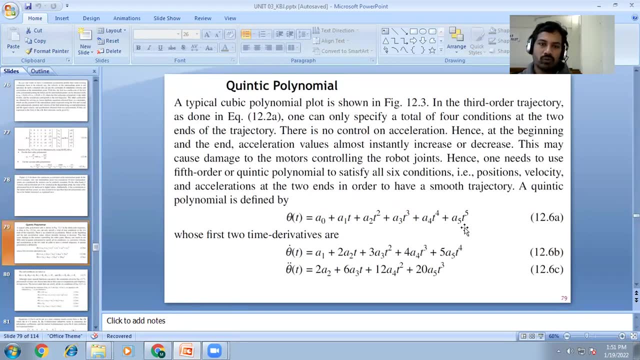 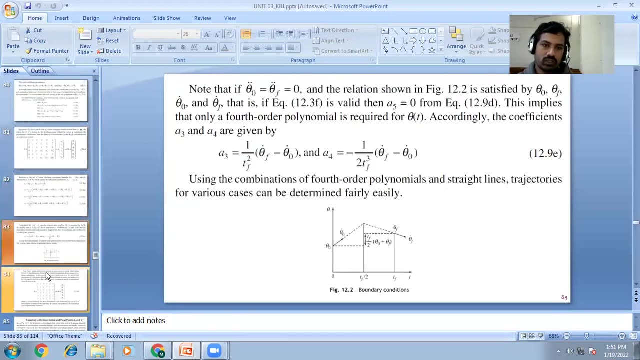 okay, just that you have to solve as a. okay, you will get that again if, having order of five there, how you can solve. okay, the methodology is given, you can go through it and you can solve the problem. okay, if they have given initial point and finaly. 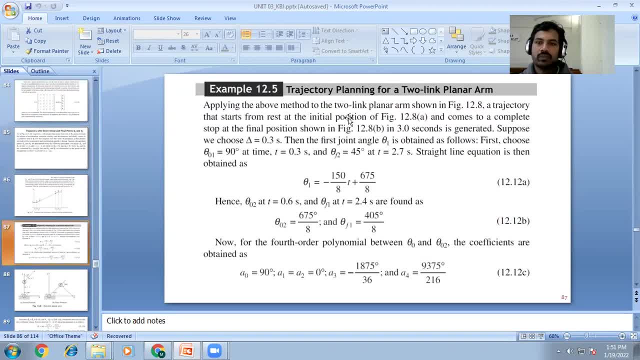 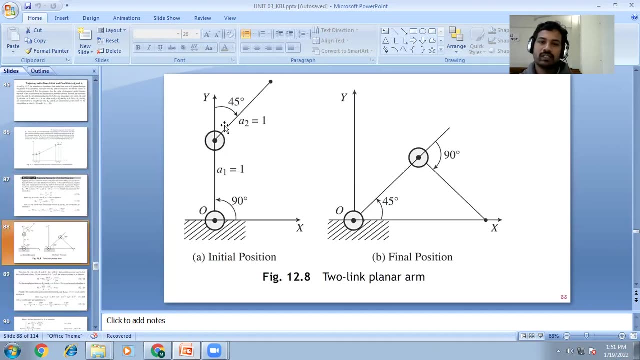 positions. okay for that. also, trajectory planning for two link planner are okay, you consist of two links. then in that case, how you can solve, okay, suppose this one is the first link and second link, and for, uh, these we want to find the angle of each joint. then how you can find. 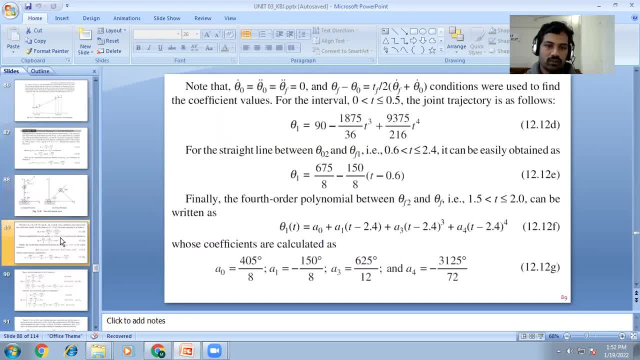 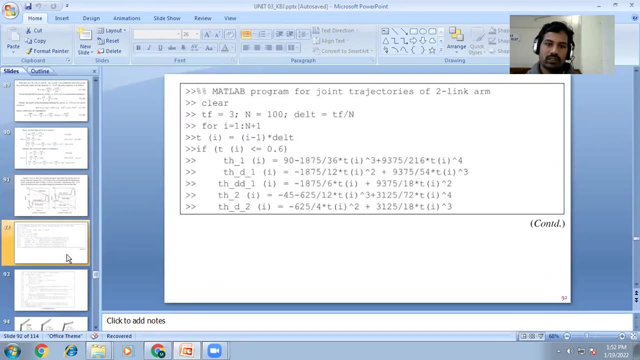 okay, you can understood with the help of this one for that, how you can take two degrees of freedom. we have to take the differentiation twice of that theta, initial and final, and from that you will find the as well as the programming also. in such a manner it is done, the programming in the define the position in matlab. matlab position to a robotic. 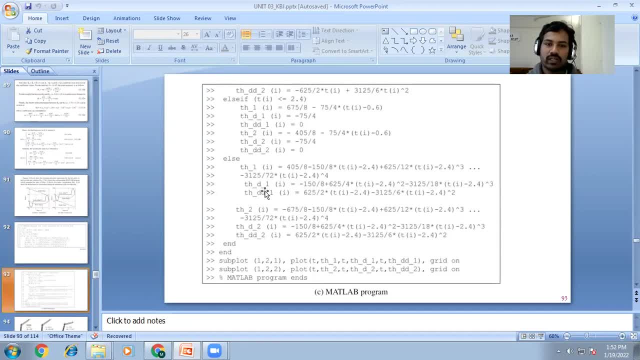 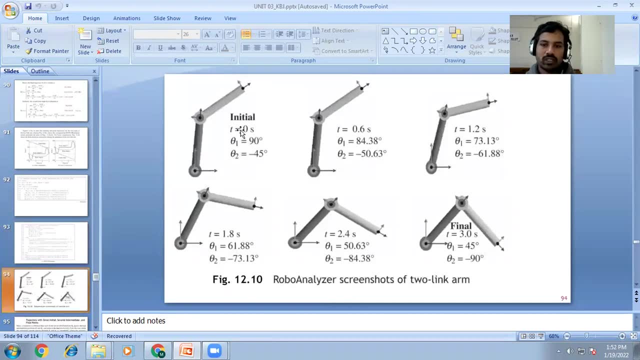 movement that he defined character cell, that you have to write the such types of program in the mat lemma. they apply. the problem means initial condition and this one is the final position to move. move this, okay, at zero, second time. theta 1 is the 90 degree. theta 2 is the. 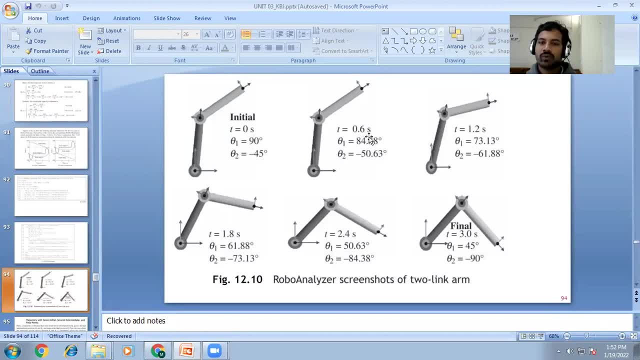 minus 45. theta 1 is the after 0.56. second, theta 1 is the 84.38 means theta 1 is going to reduce and theta 2 is increasing. man, you can see here up to the could apparently increase on either up to 90. 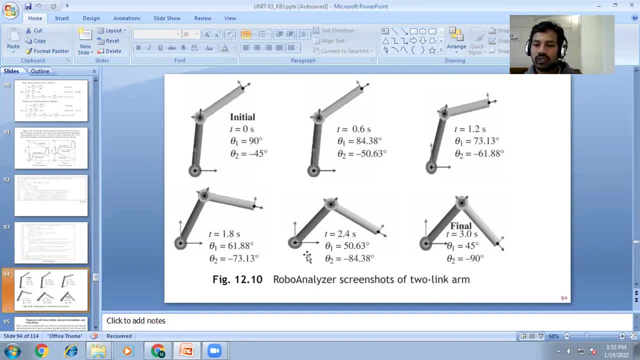 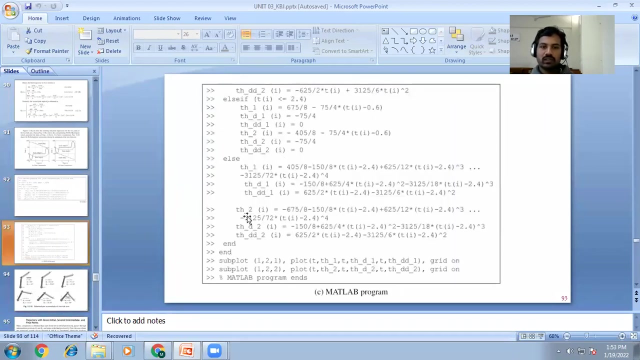 and theta 1, it is reached to the 45 degree. initial means the position at initial. such a manner after: okay, providing the timing, you will get such a position, asha position, for that you can write such a logic. okay, and from that logic the moment. so accordingly it will move that okay. next one is the trajectory with 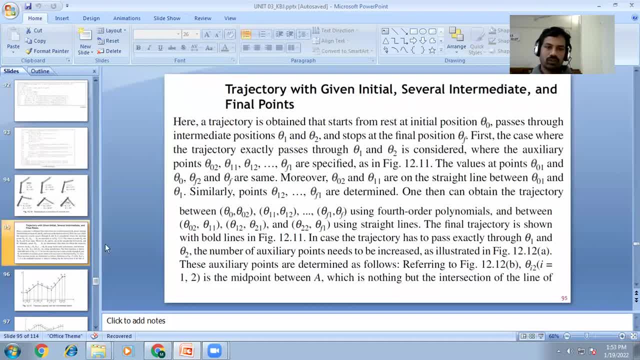 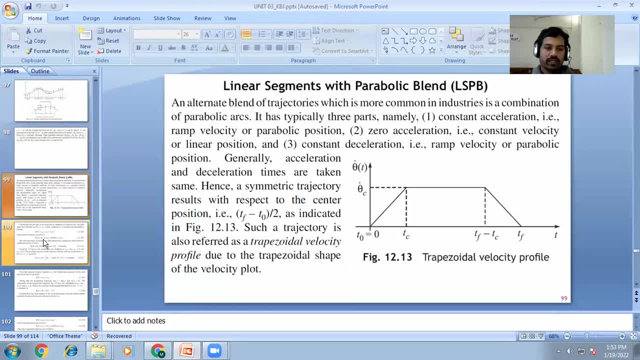 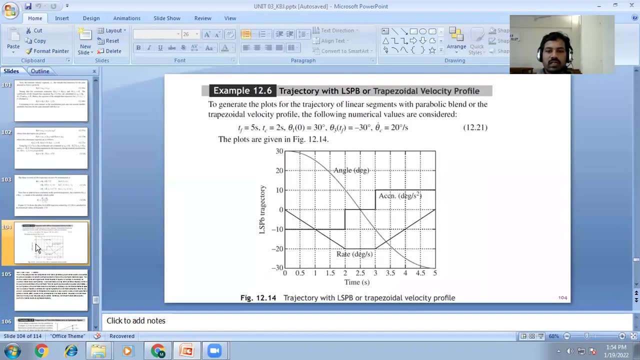 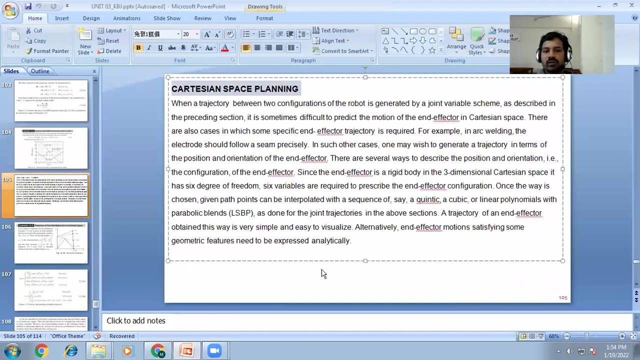 due initial and several intermediate and final points. okay, a intermediate and final point, as the case. okay, this is the extent of syllabus. this is not in our syllabus, then also, just i want to show you how that it is written. okay, now close the summer. so. 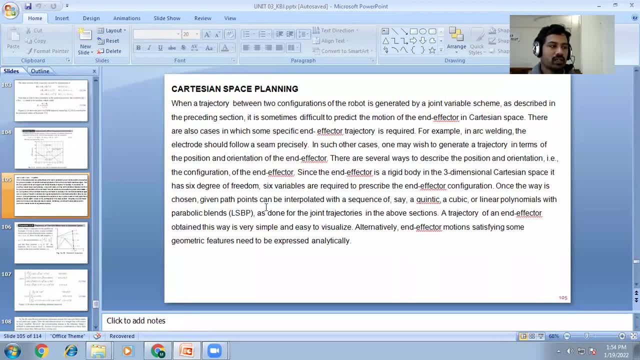 next one is the shows the the technical structure of the robot generated by joint variables, as I described in the deciding session. We can see that if the motion between base and the end effector, then we can go for the Cartesian space vector. It is sometimes difficult to predict the motion of the end effector. 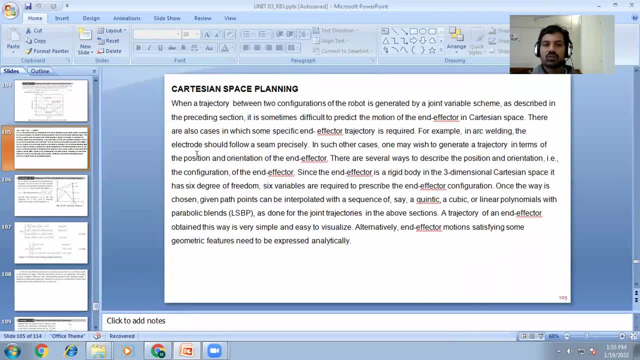 There are also cases in which some specific end effector trajectory is required. For example, arc welding electrode should follow a stream precisely. In such other cases, one may wish to generate a trajectory in terms of the position orientation of the end effector. 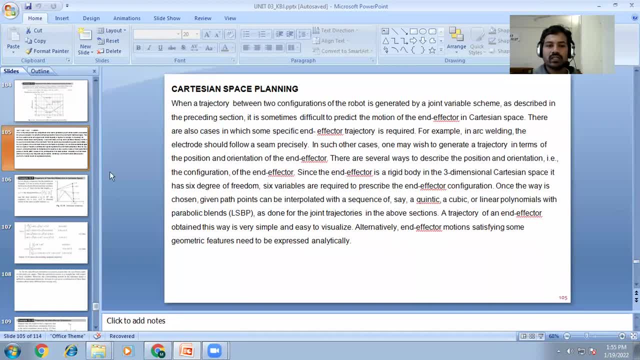 There are several ways to describe position orientation, That is, configuration of the end effector. Since the end effector is a rigid body in the three-dimensional Cartesian space, it has six degrees of freedom. Six variables are required to describe the end effector configuration. 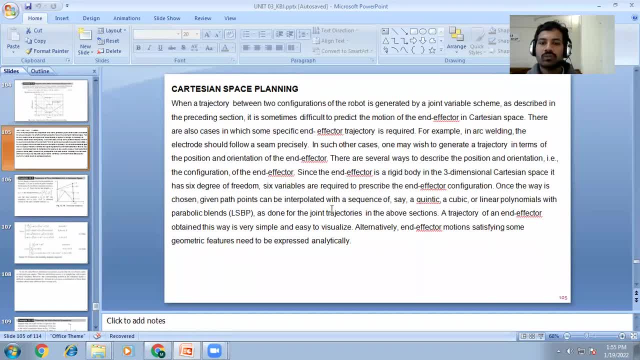 Once the way is chosen, given point can be interpreted with sequence of sets: Okay, cubic or linear polynomial with the parabolic blends, and then joint trajectory above section. This is about the Cartesian space. Okay, suppose you want to find the space. 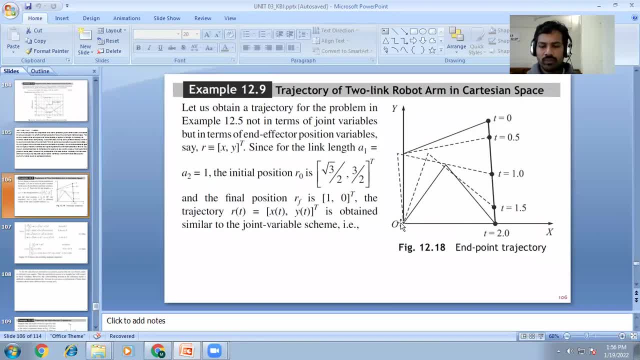 What will happen here? One will be the original base and the second will be the end effector. Suppose this base is a robot with two links. What will it do? It will find a path in Cartesian. It will find a path. What will happen? 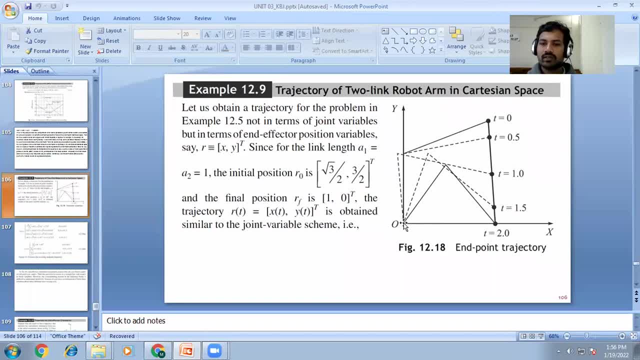 This base will be classified as zero. It will be fixed at origin And this is the movable At t time: 2.0. Okay, let's say two points. Yes, it is an X axis. After 1.5, it will reach here. 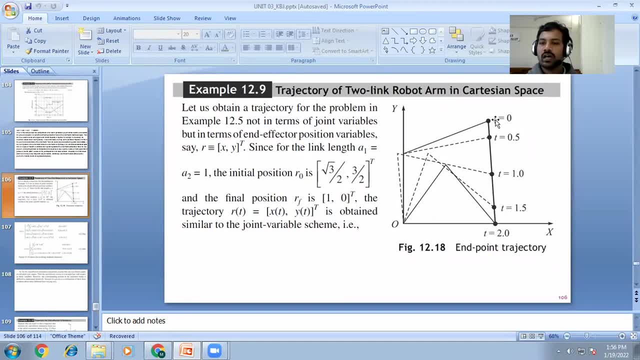 Suppose, at the initial our robot end effector is here, Then as time goes on, increasing, you can see here The motion of the this t time is increasing motion of each link particular motion. it is not in this Cartesian we are not discussing. 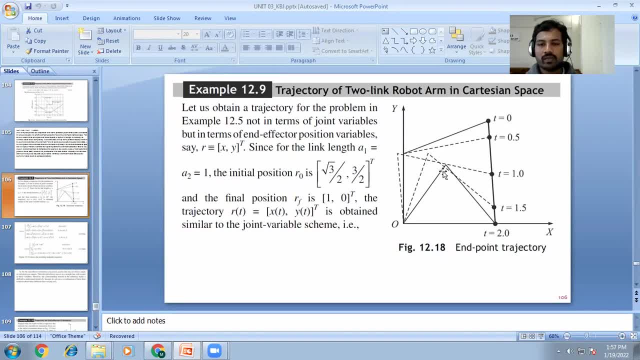 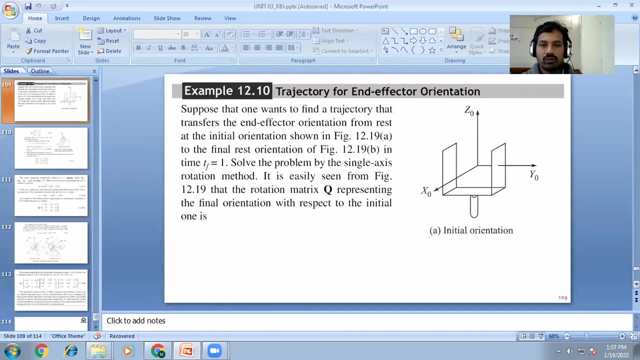 about this. angles have done the link model of the angle. I have a drop on. can he- which I couldn't have had done- link model to end effector. on a base model, a machine motion, a 30, 30 can happen- find out? this is the sum of the power formula. from that we can find: 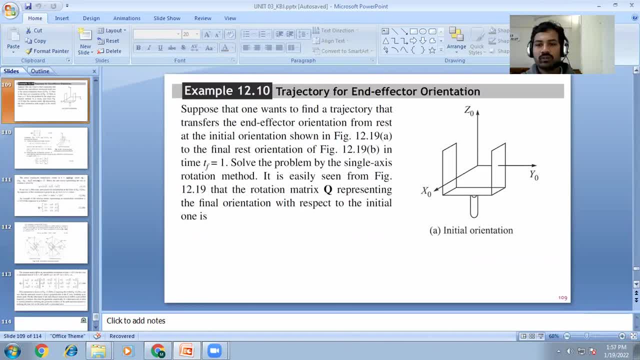 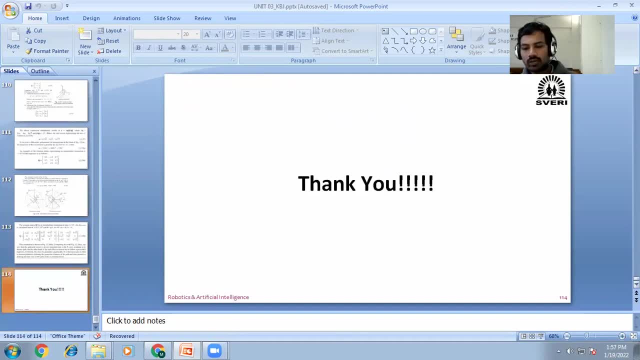 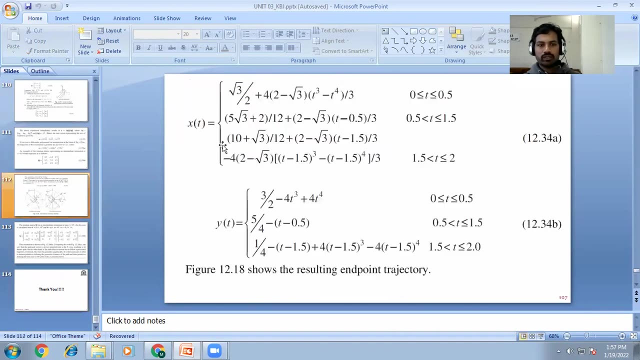 out trajectory of end effector orientation. okay, how would that find out? we will find out with these formulas. where this is about the, our third unit, if you have any problem in this unit you can ask directly to me. they have a day at three unit money when our problem. 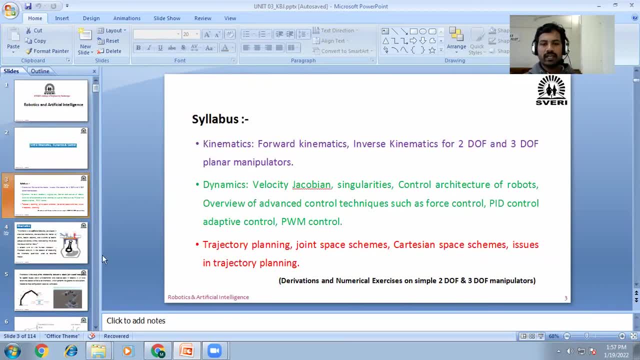 center, which are sector about the kinematics, dynamics and trajectory plan. we have covered all points from this tree. Okay, most probably today you need- I will share one test on this, our third unit- to say you need to take this to share curry. you have to solve, sorry, you have to solve that. 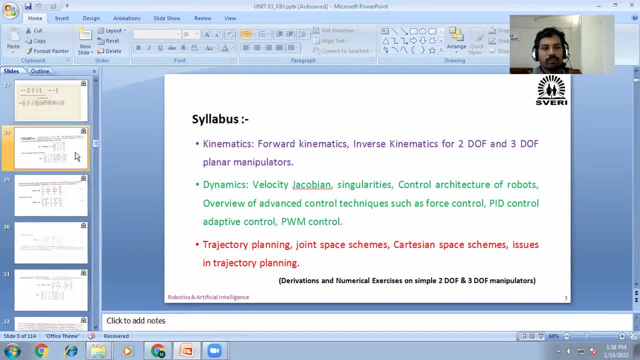 test. okay, because mostly numerical part on. if you see our whole syllabus in third unit only you will find the numericals and other units are. it is a related, only theorem. Okay, You have to see the sum of the formulas and the problems it is related to only forward. 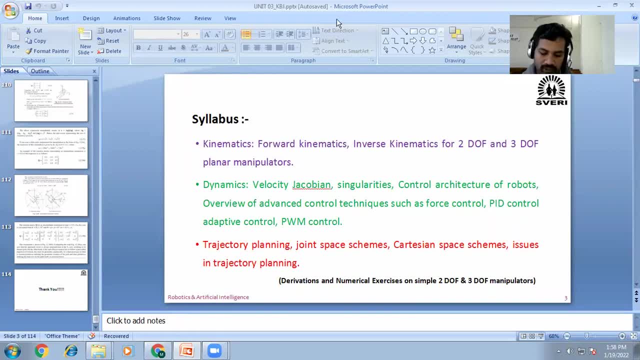 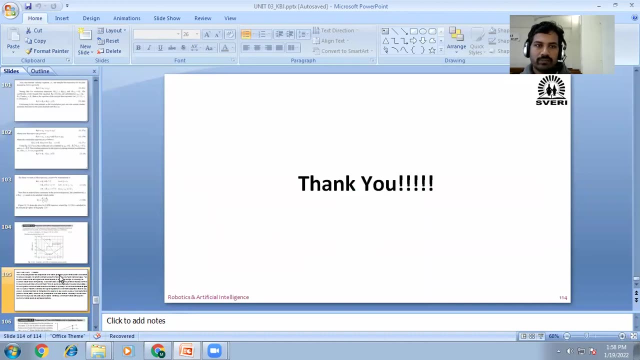 kinematics, inverse kinematics, forward, any inverse kinematics with the list to multi decany problem but other. there is no any problems in this subject. okay, if you have any problem you can ask up to the trajectory. okay, All syllabus Are completed from my side. give my just sign up for the order, kind of point cover cut. I. 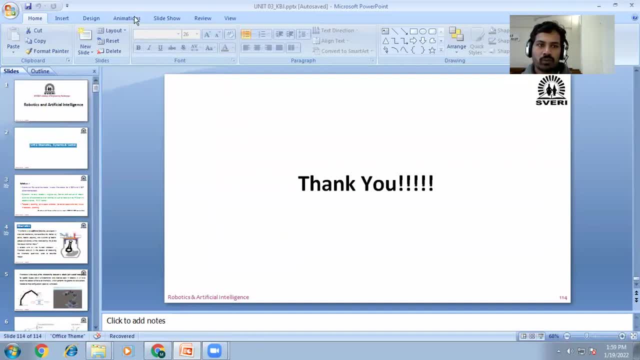 will give this a great point. me cover, Kelly, like if you have any problem queries here after, you can call me, and for paris you can ask me. okay, because the problem queries are saying that up there, robotics with the call for which are we set up? I am ready to give. 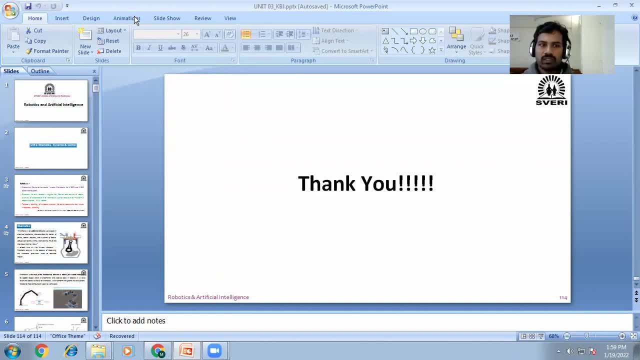 the answer related to that. now, This Is End of our robotics and artificial intelligence. and one more request from my side: all are requested to write the assignments, which is I have provided six assignments, how to complete that assignments and you have to upload on that submission link as early as possible. and one more instruction: 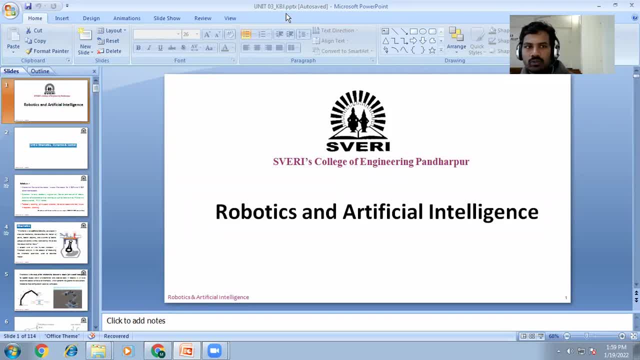 from my side related to exam form. Okay, Those how yet Not To Fill the exam form. please fill it on our agenda basis, because exam will start from backlog. exam will start from 24th to the 24th person exam start. owner. a third asset is a granular 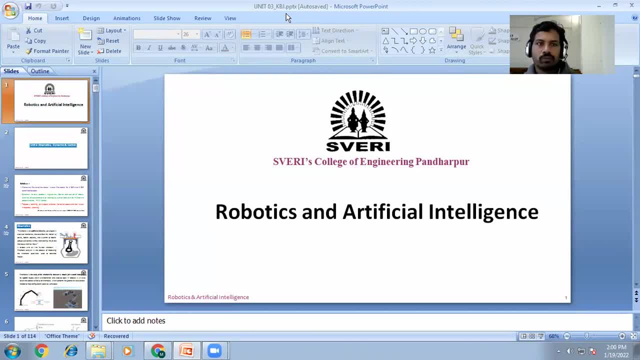 occur at local Jennifer Leland center. can exam form Philip gonna? okay, this is from my side. we are all about the robotics and artificial, as well as the from instruction. okay, administrative instruction from my side. Okay, If you have any queries, you can unmute yourself and you can ask. otherwise will end our session.